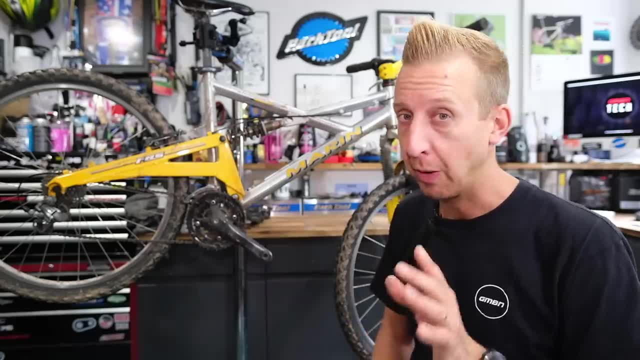 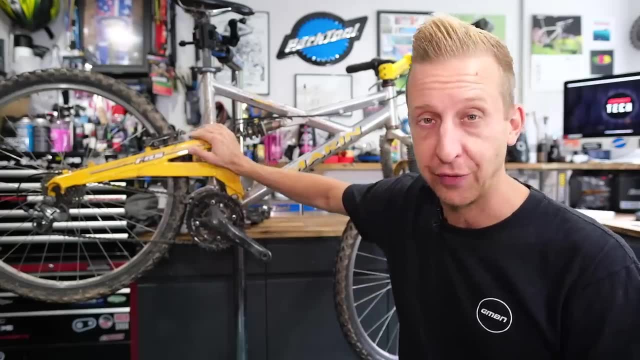 good option here and well worth spending the time on. Hopefully, we won't need to spend any cash on it and, if at all, a minimal amount. Now, Blake used this for a presenter video where he spent 100 quid to buy the thing, so he got it for a bit of a bargain As a result. 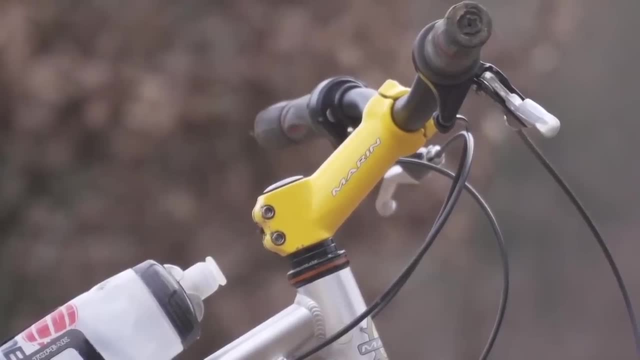 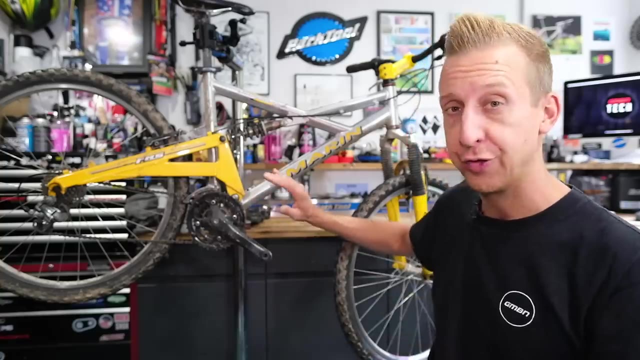 we absolutely trashed it. It's been at the back of the GMBN lockup, which is where we found it, amongst other terrible condition bikes, but I thought this one was a really good candidate. Reason for that is it's got a bit of history: Marin bikes in the UK. they're massive. 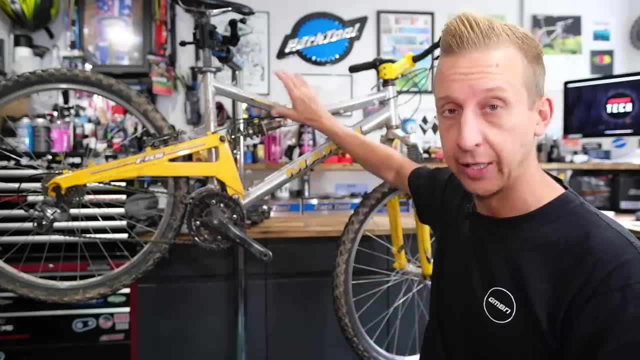 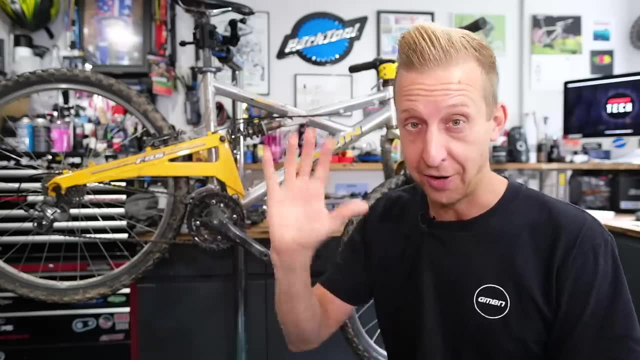 everywhere, but in the UK they have a real cool story. In 1996, they had a cross-country version of the same frame layout as this, called the Mount Vision, A guy called Paul Lazenby- if you're watching this, Paul hi, I know you watch the channel- absolute legend. he became the first. 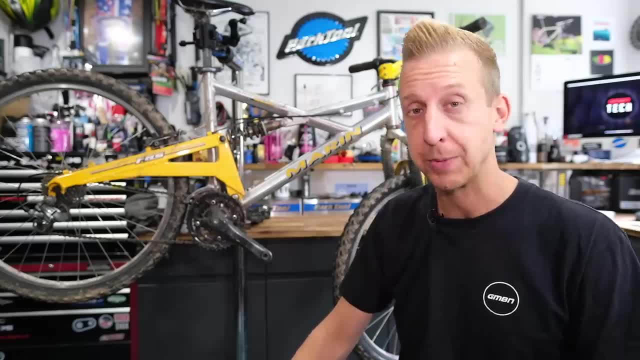 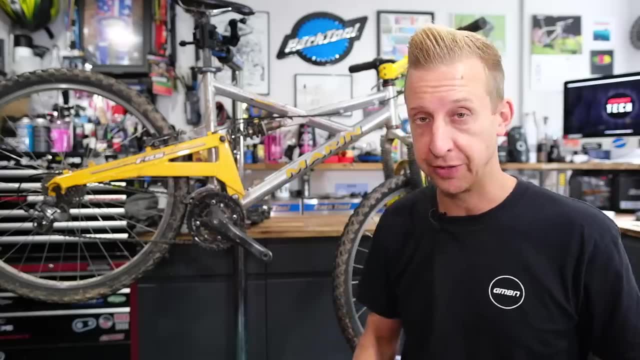 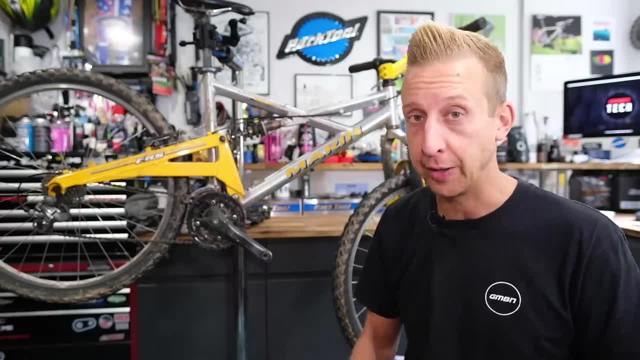 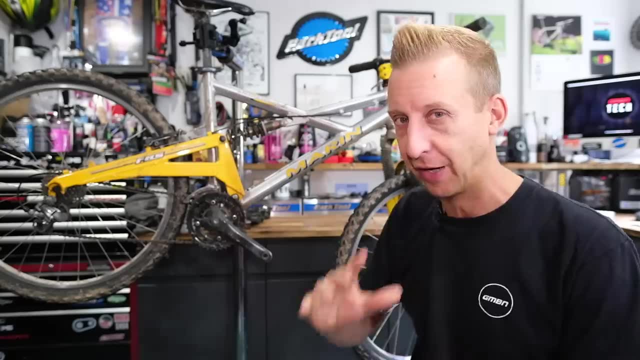 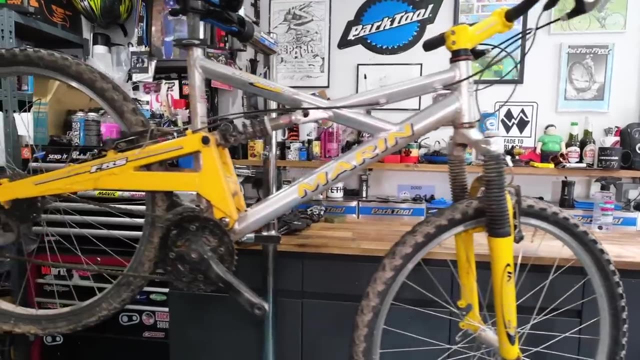 to going faster. He really opened that up for everyone and really put Marin out there in the limelight. I think it's really cool. This nods back to that. I think it's definitely worth doing the bike up. Let's have a little closer look at it, shall we? 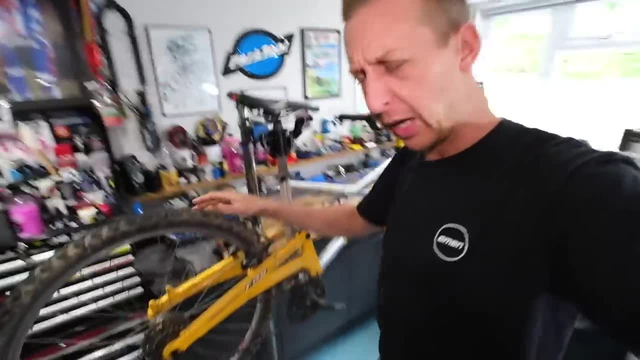 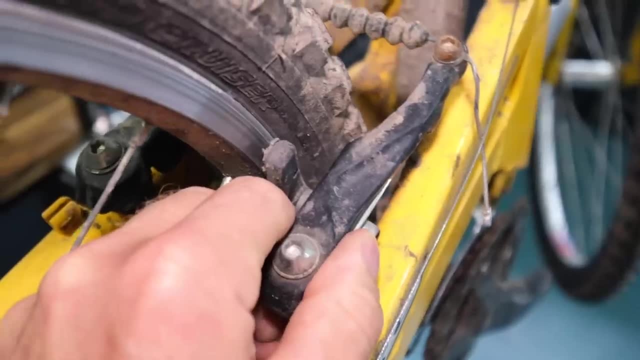 It's obviously filthy. We're going to need to give it a bit of a clean. Rear tire is flat as so. I'm guessing it's got pinch puncture Rear brake blocks- they don't even touch the rim- Always a little bit of a concern. 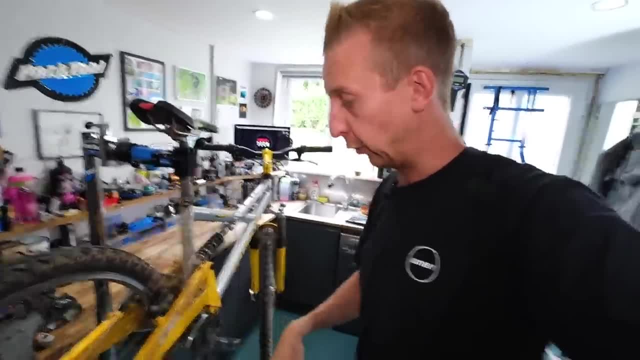 We may need to replace the brake blocks, but luckily they're dirt cheap. You're talking like probably four or five quid for a set of brake blocks like that. That rear derailleur's all over the place. I don't know if you can see that down there. 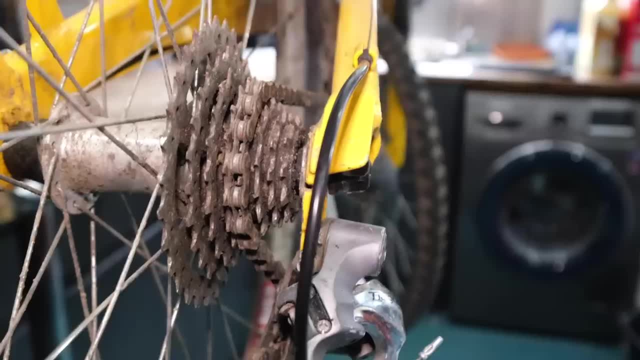 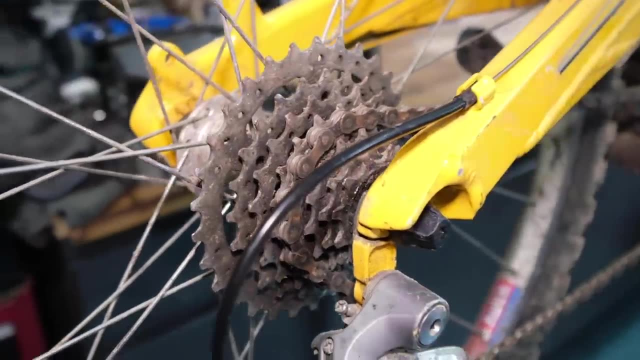 That has had a hell of a whack at some point. Yeah, that's not even straight, so we'll bend that back, Something that's quite handy about older bikes. so this one's got eight speeds on the rear and three on the front. 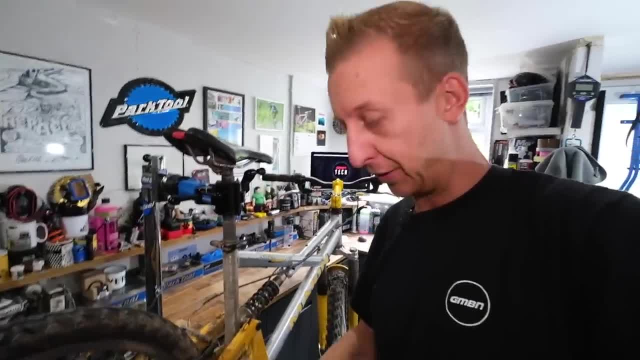 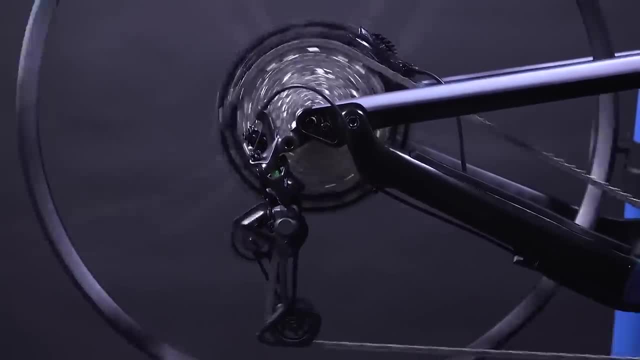 The fewer gears the bike has, the easier it is to get them working again, because of the fact it's not so precise as the really cool 12,, 11, 10 speed stuff we have today. That stuff has to be perfectly aligned. 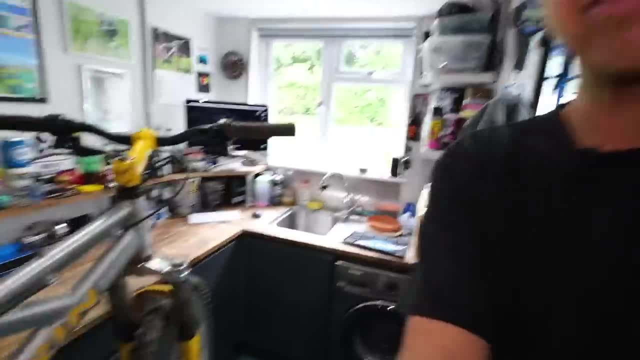 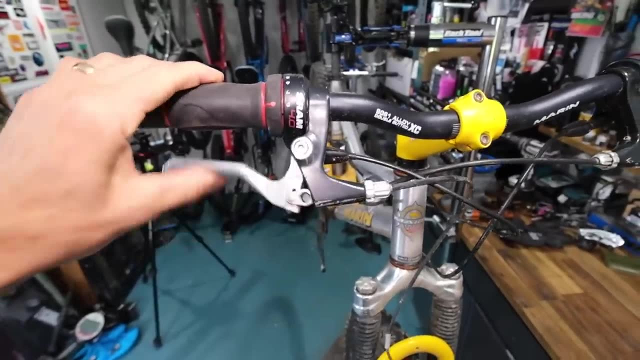 This stuff far less so, so a lot easier to actually fix up. Okay, so, moving on to the front of the bike here, Let's have a look at the handlebars. So oh, that's a little bit sticky. I don't know if you can see that. 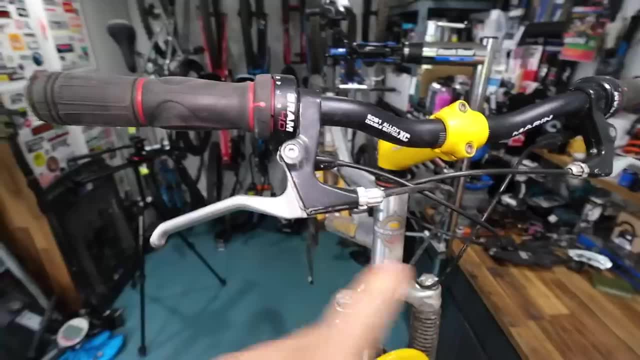 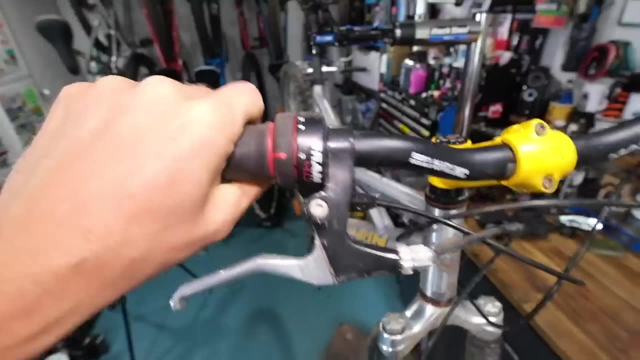 It wants to stick. so we will take the cable out and we'll give that a good bit of lube Shifter, Little bit sticky. We can make that work a bit better. The other brake lever, yeah, all the way to the bar. 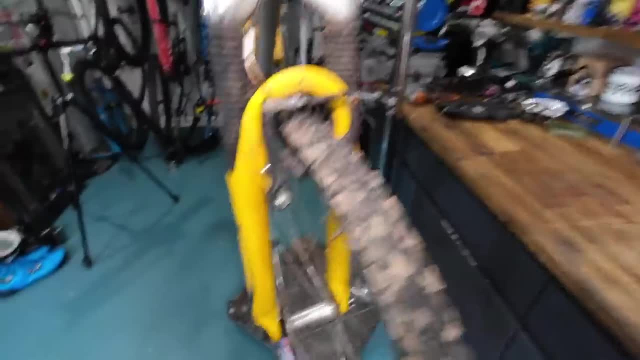 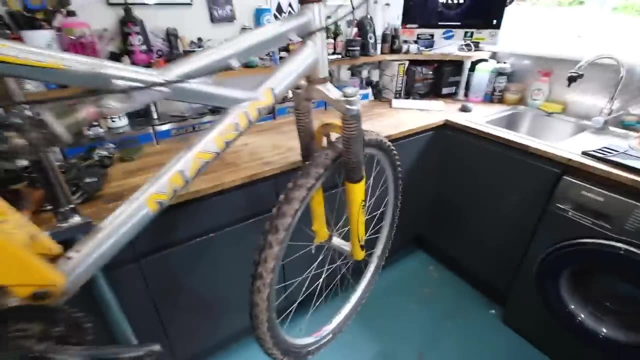 so we'll need to sort the cables out on that. Obviously, give that a safety check up at the front here as well. Front tire doesn't look too bad. Little bit perished though, So something with tires The longer a bike has been in storage. 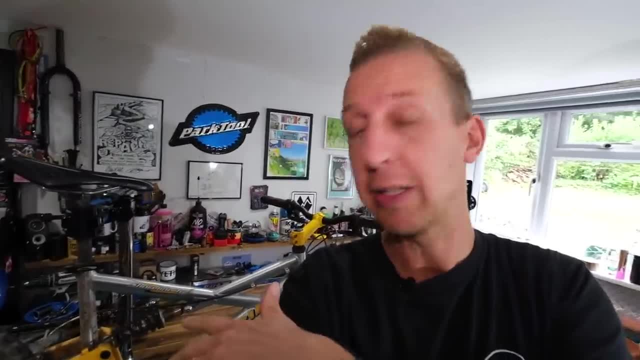 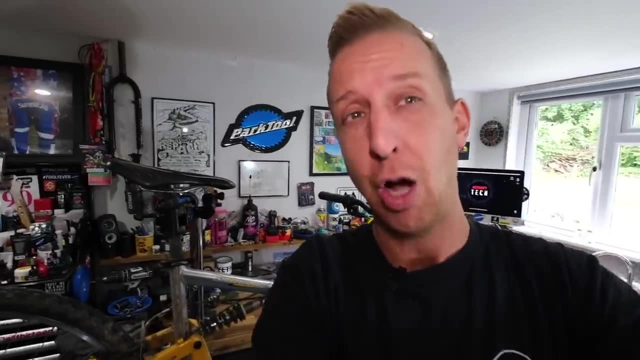 the more likely it is that you're gonna need to replace the tires, But luckily, being 26 inch, you can get bargains on them. I reckon I could pick up some tires for less than 20 quid for a pair, So hopefully that's really all we need to spend. 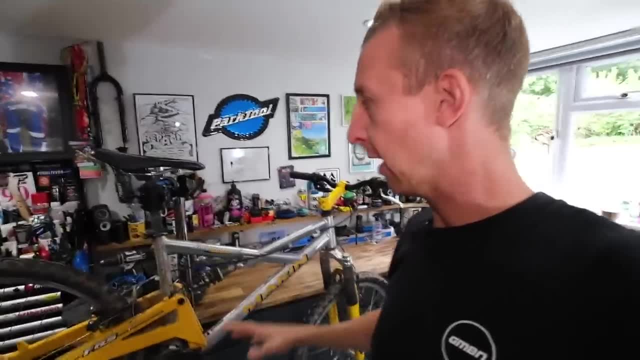 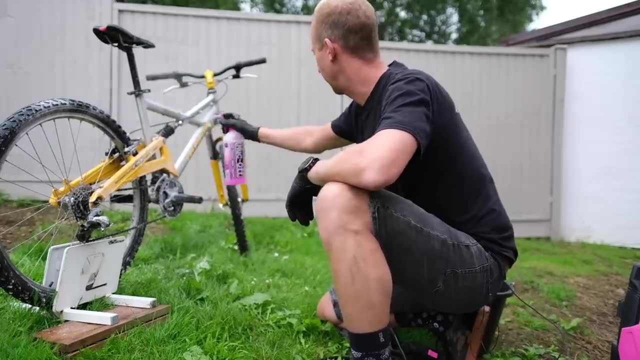 Perhaps brake pads and perhaps tires, But that's it. Let's give it a bit of a clean, shall we, And then we can actually see for sure. Okay, so I'm using some proper bike cleaner on here. You might not have access to that. 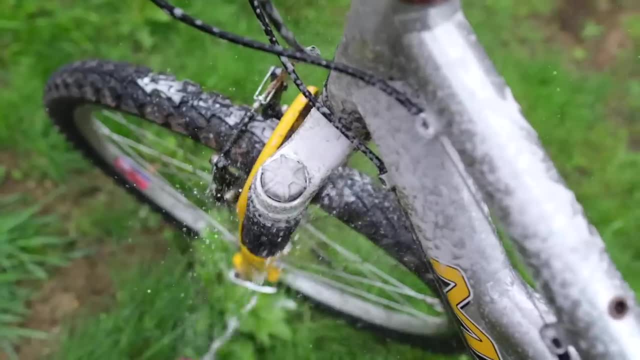 You might just have a simple bucket and a brush. That will do to get a bike clean, although you really can't beat this stuff. I've also got the luxury of having a jet wash, so I'm gonna get this hammered out quick. 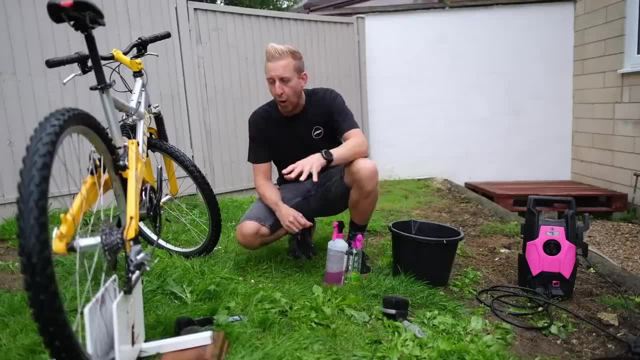 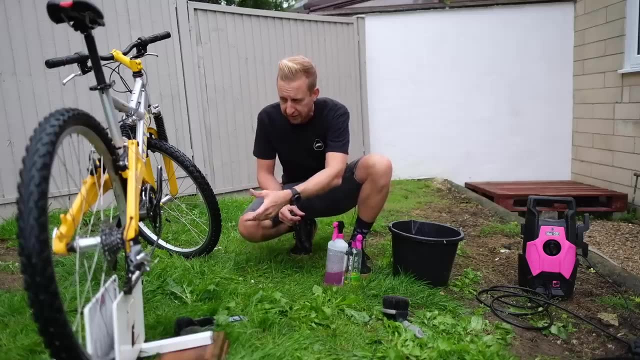 Okay. so normally at this stage I'd be telling you to give the bike a bit of a wipe down, because you really want to clean, protect and then lube it. Protecting, of course, means using a corrosion inhibitor to drive out the moisture so you don't get any rust. 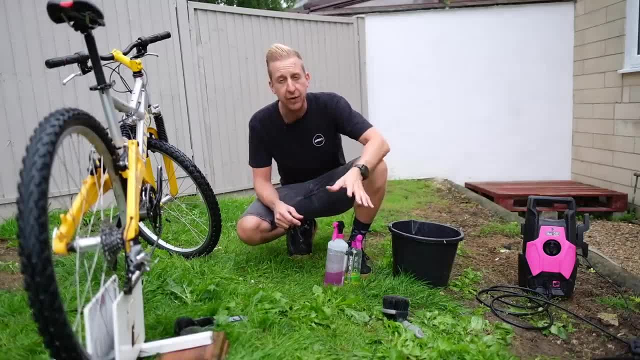 This bike has already got a bit of surface rust on the chain. However, given the fact we're doing a bunch of other things to the bike, I'm gonna take it inside, let it drip dry and have a cup of tea while it dries off. 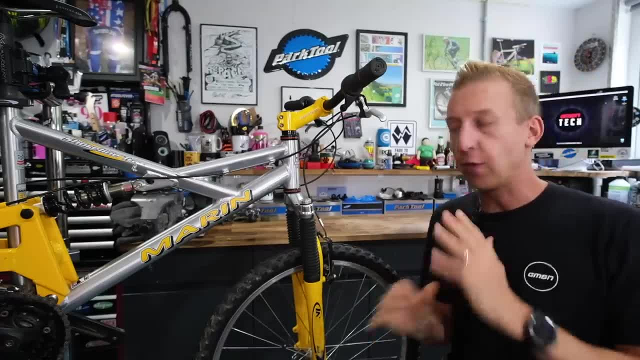 Right, okay, so the bike, as you can see, is looking a bit cleaner. Now, before we get started on it, it's important to make sure that you've got a clean bike. It's important to have a sort of method. 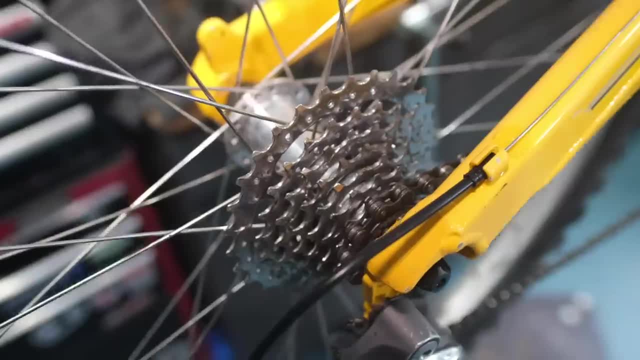 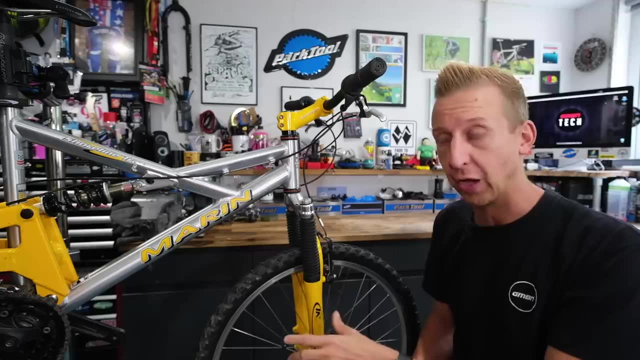 however, you're gonna work on any bike. I'm gonna work front to back on this one Now, when I was inspecting the tires on it as I was washing the bike, I did notice that there is a bit of a slash and a sidewall of the front tire. 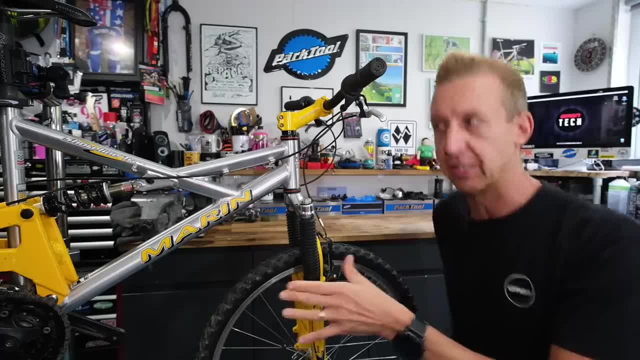 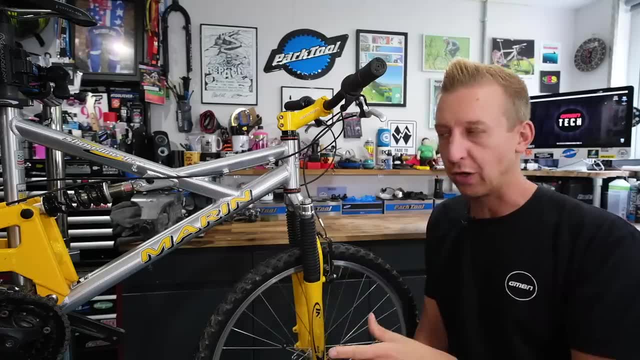 I inflated them and they're both still kind of up, so I think it might just be a slow puncture. so I'm gonna take my chances with that. but I am gonna swap the tires out Now. I could order some, but I do have some tires. 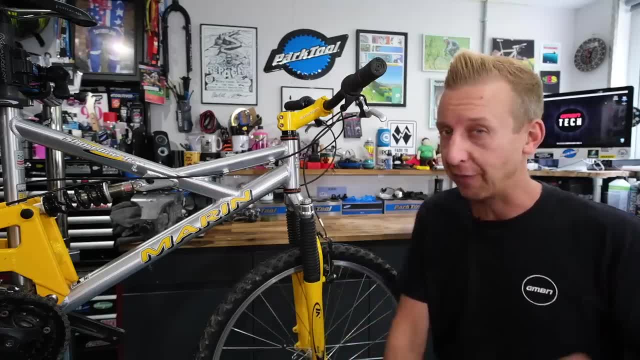 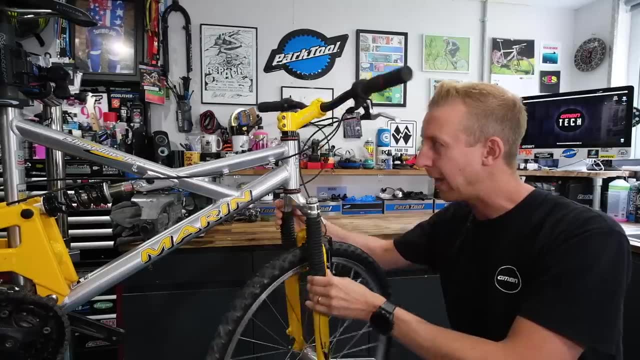 that won't go with this very well up in the loft intended for another bike, so I'm gonna actually chuck them on here for argument's sake For the time being. So first port of call is to check out this headset. that sounds a little bit notchy, but it's not too bad. 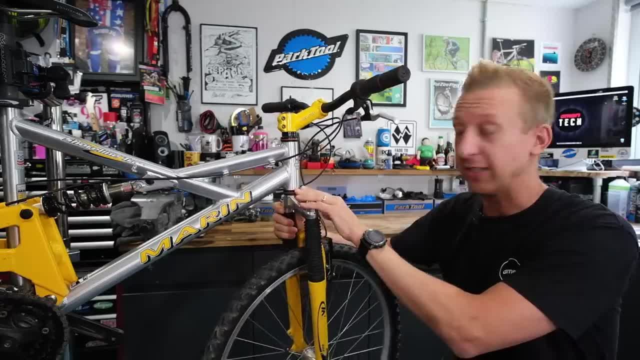 I suspect it's just got barely any grease left in it, or any grease in there is a bit manky. So super quick and easy to do that and then the front end feel nice and then we're gonna get the wheels out. 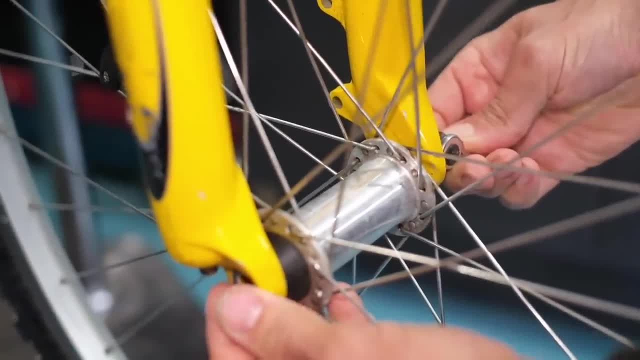 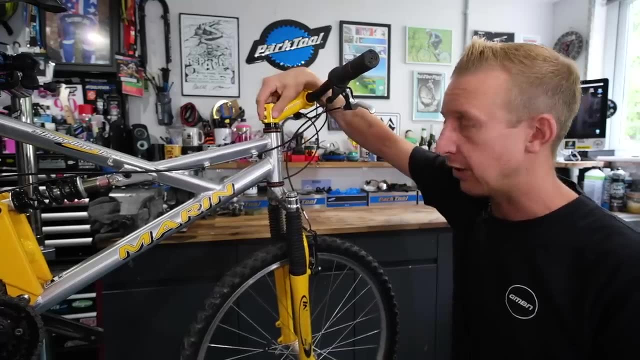 swap those tires over, then I'm gonna check out that front brake and make sure it's nice and safe and it works like it should do. You wanna start by taking the top cap off, or at least loosening it? Then you loosen those stem clamp bolts. 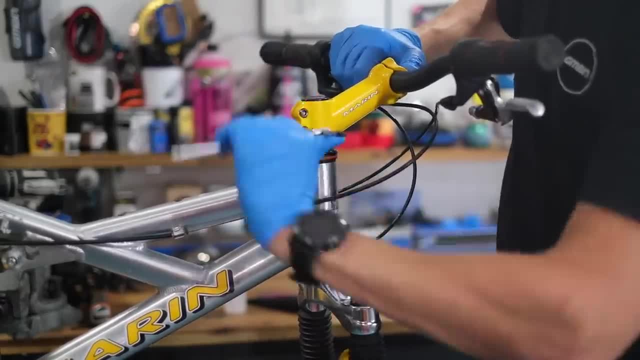 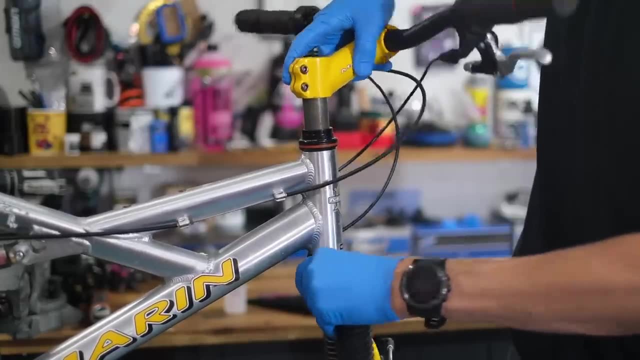 Once they're loose, the top cap is the only thing that's gonna stop the stem coming off. So make sure you hold onto the fork, release that top cap, wiggle that stem off and let it just dangle carefully, and then hopefully you should be able to slide the fork out. 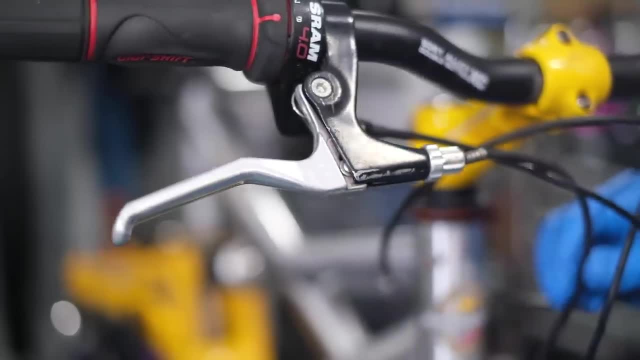 Now, because I wanna slide that fork out. you're gonna need to disconnect the front brake. You could take the cable off the brake, but actually, because these are old cable brakes, you'll find there's a little slot in the barrel adjuster here. 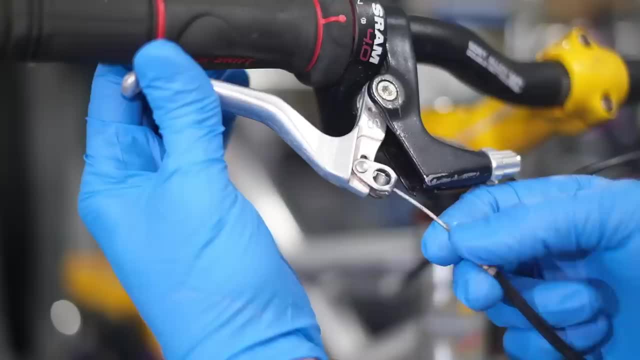 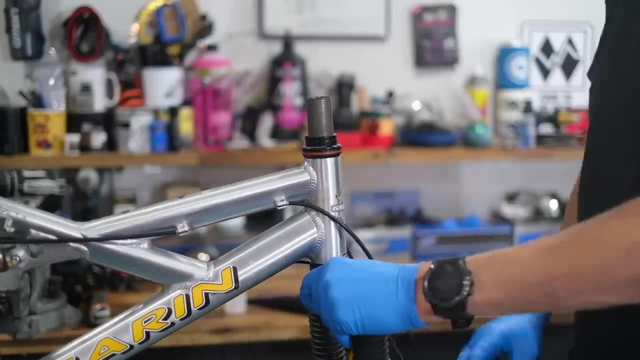 and if I just slide the cable out the side of the bars there, you'll find that you can actually disconnect it at the lever. there we go. So there is that cable Away Now, like this bike that's been around for. 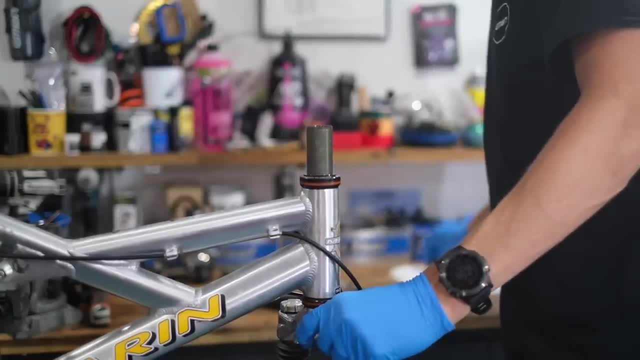 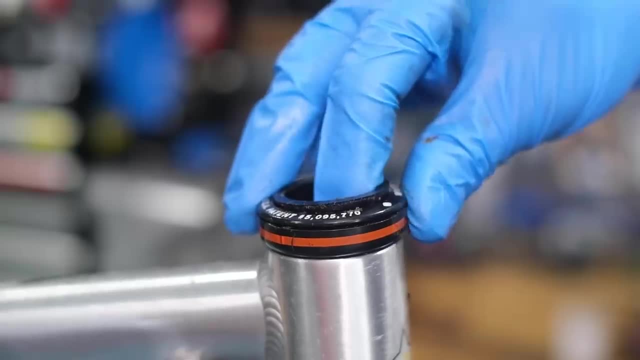 well since 2001,. I suspect this has never been done on here. You might even need to tap the steerer tube just to get it out and free it from the system. Now, as you can see, it's pretty gunky in here. 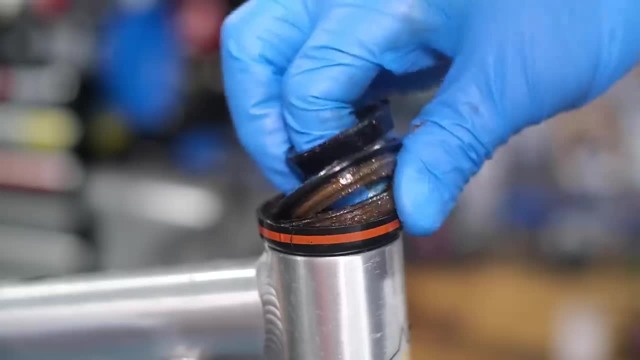 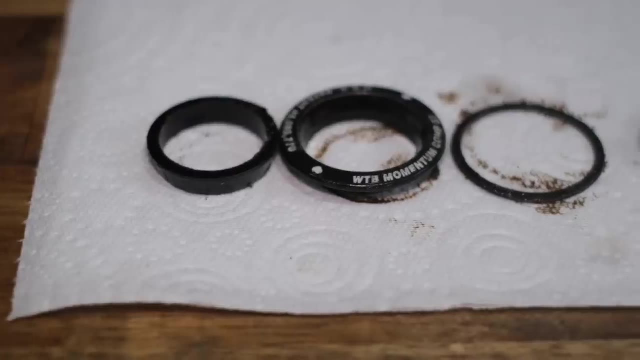 So if you're gonna remove any parts on a bike to clean them, put them down, ideally on a workbench or a working top, and you want some sort of shop towel or some kitchen roll, something like that, so they don't roll anywhere and you can just use that. 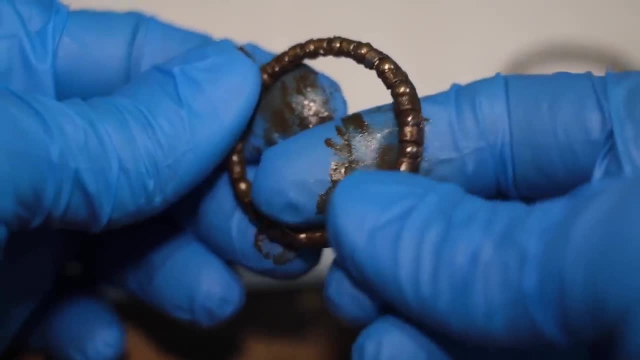 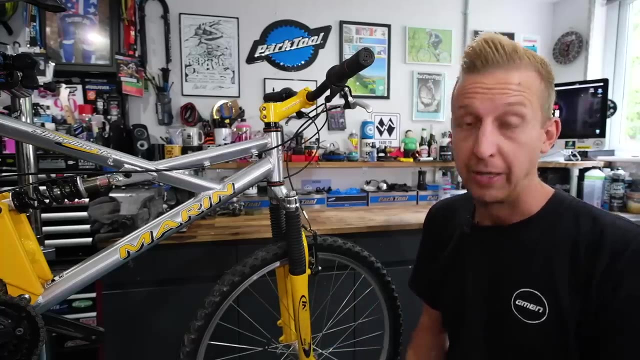 to clean them with. at the same time, Again, it's always nice to use some proper cleaning products. You know, I'm lucky enough that I've got everything here at my disposal. but you might not have, So you can use some. basically just a bit of elbow grease. 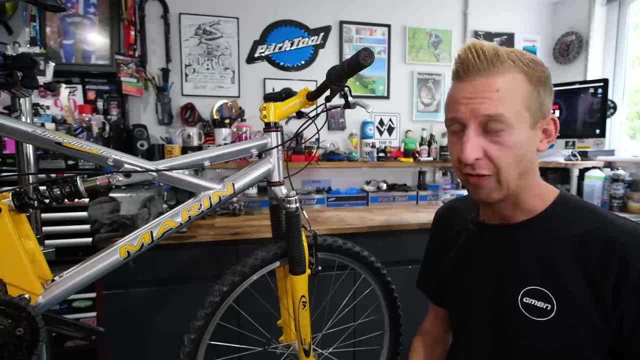 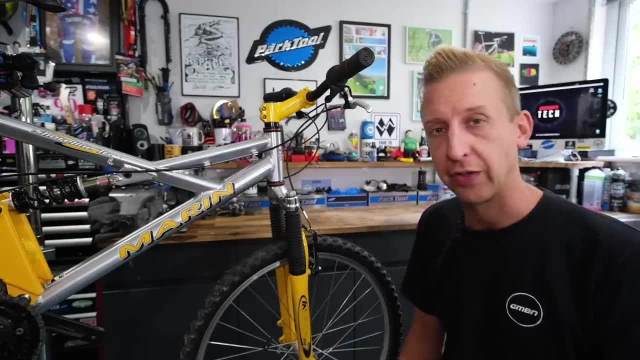 If it's really mucky you can use things like household cleaners and stuff. but to be honest, you want to kind of steer clear of that stuff. if you can, Better off just using a bit of elbow grease. get that stuff nice and clean. 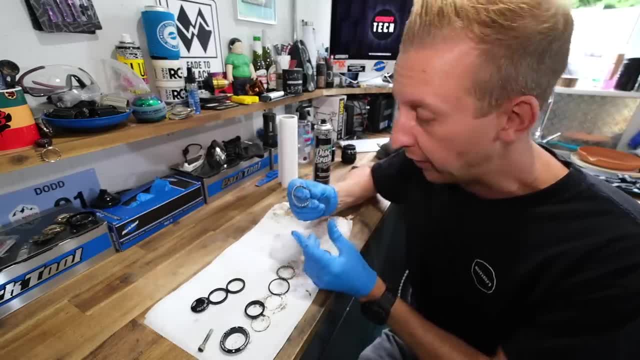 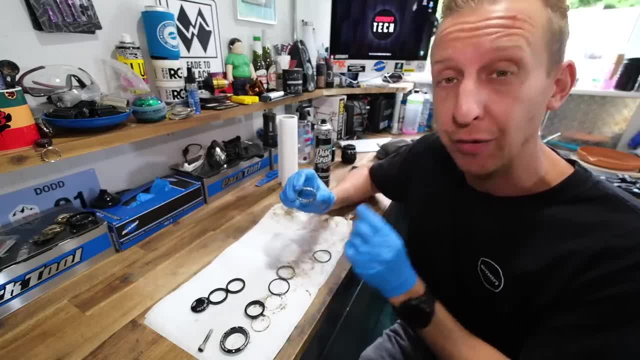 so you're gonna find bearings similar to these. so you're gonna find bearings similar to these- bearing similar to these- on a lot of old bikes, which means they're really easy to clean, provided they're not too worn out. These are actually in excellent condition. 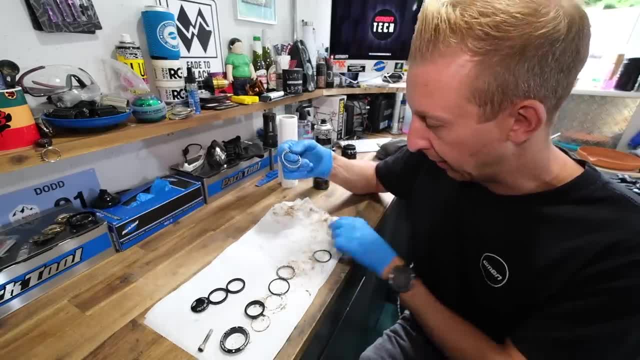 they just needed all of the sort of crap flushing out of them. You can see about the state of the rack here some of the color of stuff that's coming from, So these will be great. just let the isopropyl alcohol. 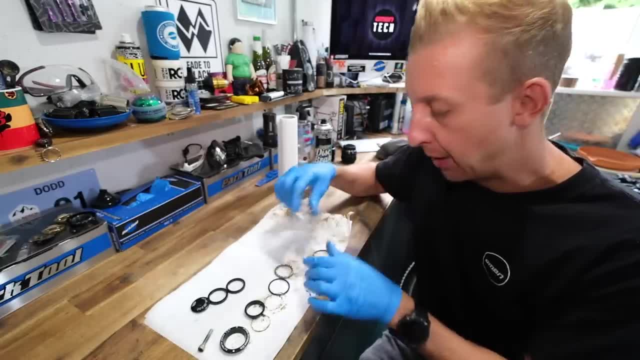 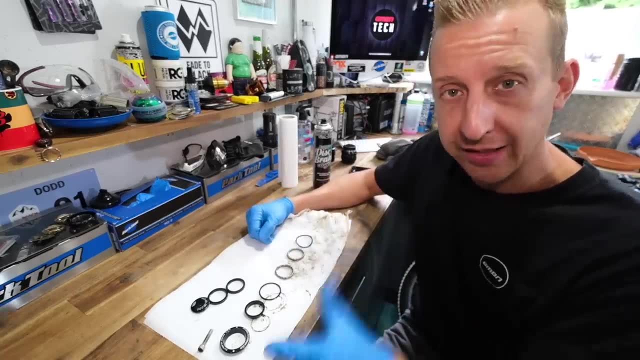 on that disc brake cleaner, dry out completely before I think about putting them back in. In the meantime, I'm just gonna give the frame cups a wipe down and put some fresh grease in, then this headset back together and that's that bit done. 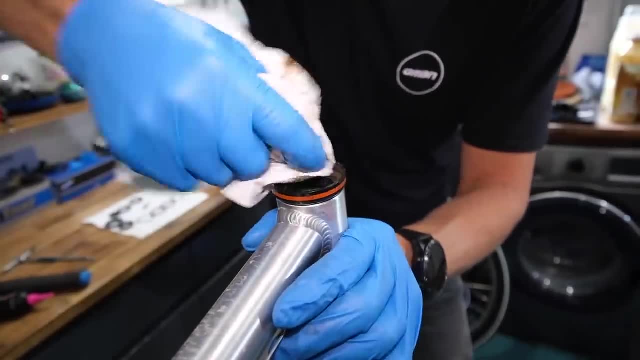 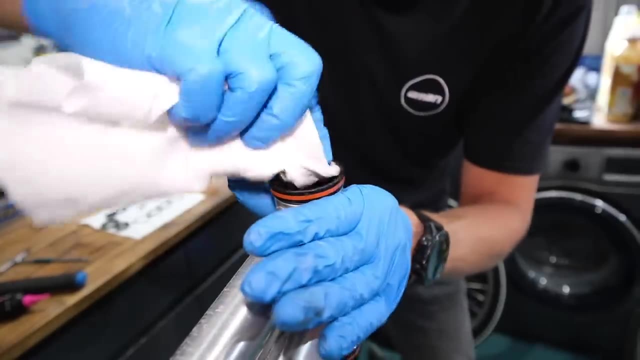 Now, something I probably should have said is, when you're cleaning out these cups, just give them a little feel with the ends of your fingers. Note, I'm using gloves because these are really gunky. You don't have to If you're old school and a bit of a mechanic. 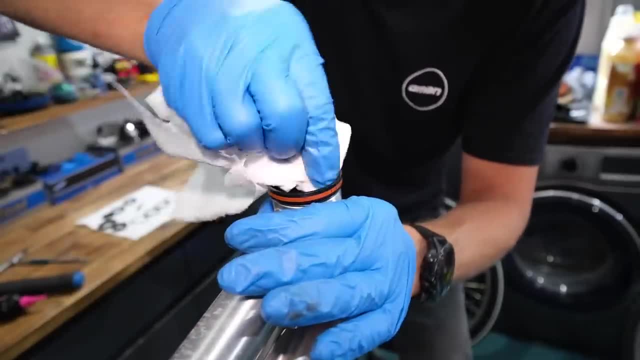 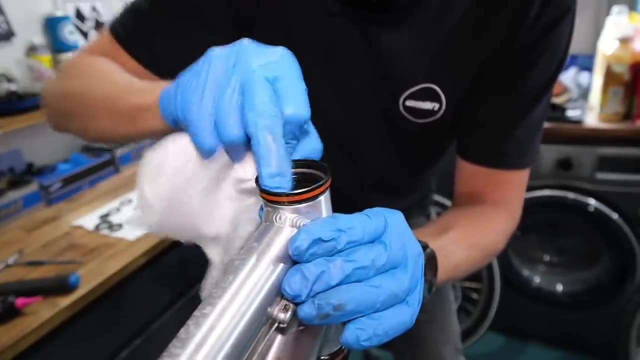 use some barrier cream on your hands before you do this. That way you just make sure the grease doesn't soak into your skin and it means they're gonna be easier to clean afterwards. Yeah, look for a nice smooth bearing surface if you're using traditional bearings like the ones I am here. 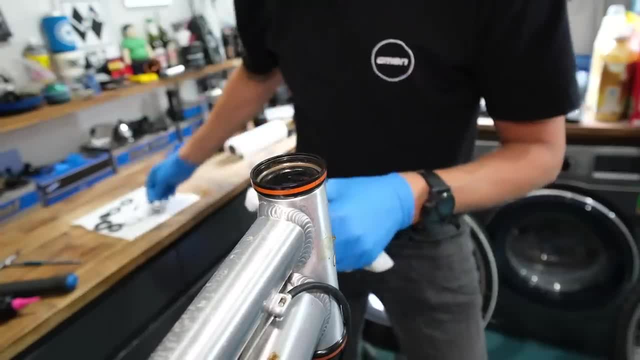 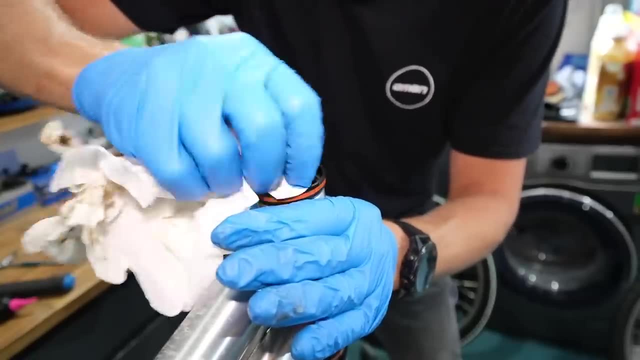 because you want them to spin nice and freely around here. If those bearings have been worn or the bearing surfaces get pitted, that's when it's time for a new headset, and then you're gonna have to reassess whether it's worth it on that bike. 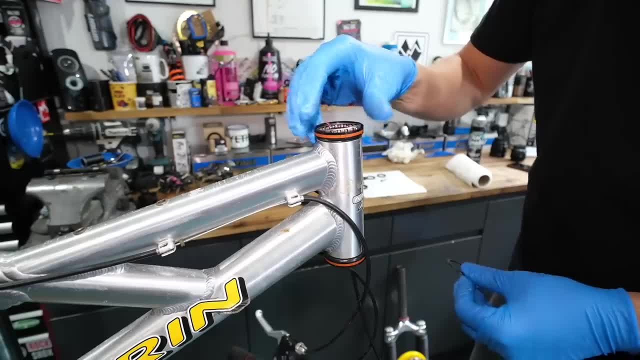 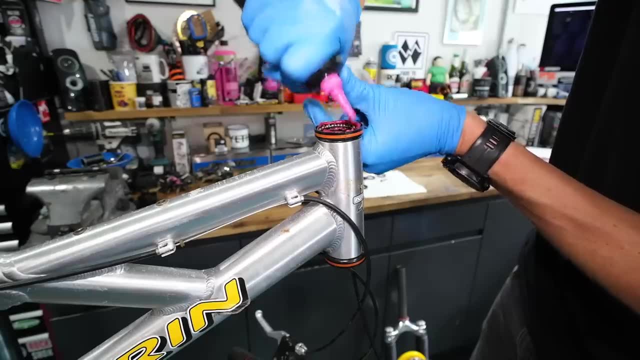 There's no substitute for having a good quality grease, though, for your bike. Now there's lots of different greases available to put in different parts of the bike, but a good general purpose grease that is carbon safe is a really sensible thing for you to have. 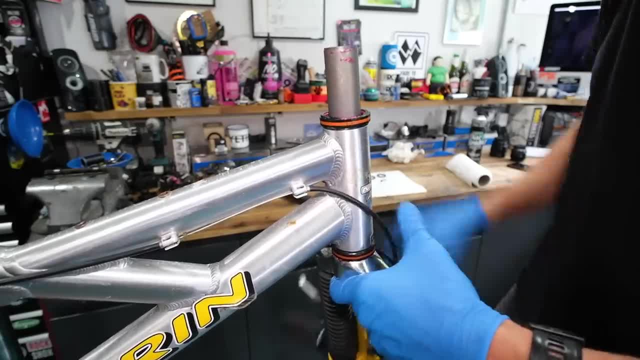 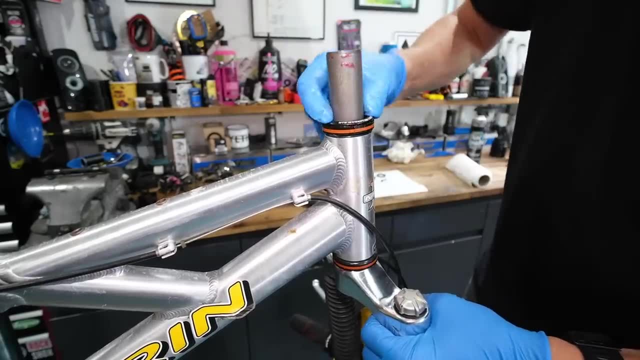 in your own workshop. Okay, pretty simplistic here, just sliding the steerer tube back in place. I'm gonna make sure I wipe off the excess grease afterwards, and I might actually use a bit of isopropyl alcohol or disc brake cleaner. 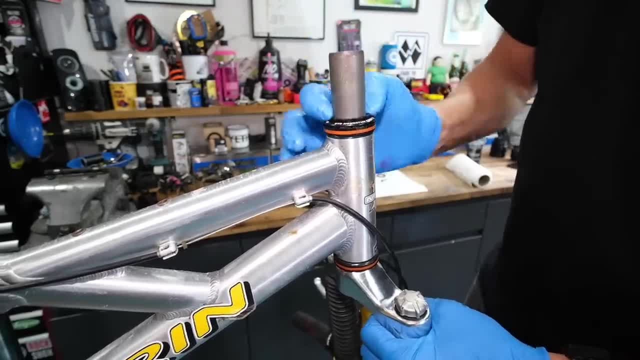 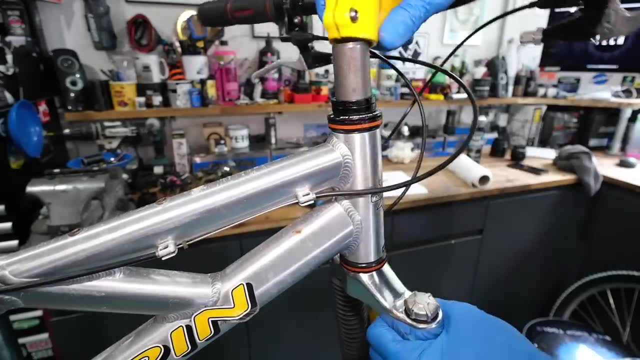 on a rag just to make sure there's no residue on the frame and on the outer cups of the headset there, because that's where dirt and grime will stick afterwards. Just a little tip for you there: Put it back together Before I clamp the steerer tube up with that stem. 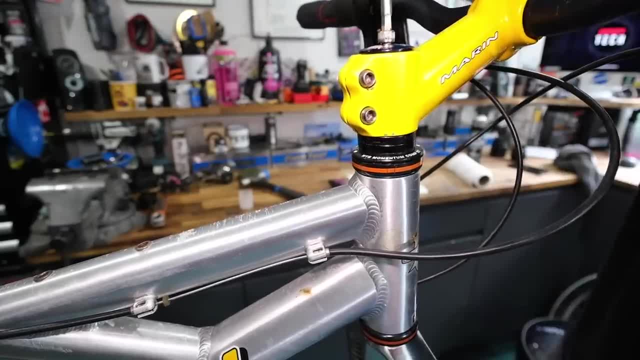 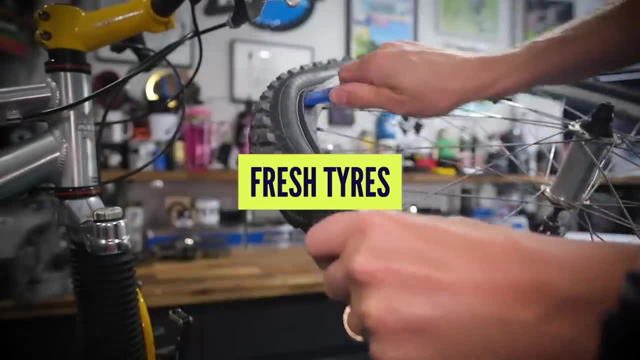 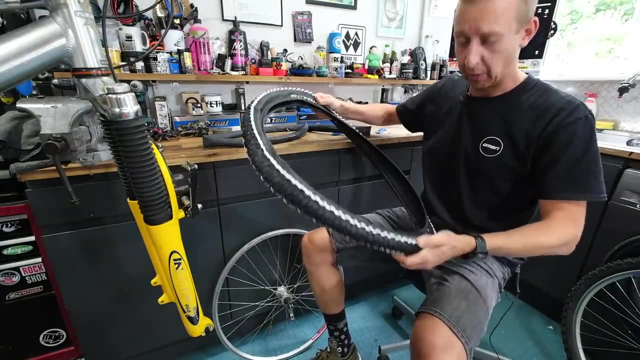 I'm just gonna adjust the top cap there until the headset feels like it's running smoothly. but there's no play in it. You clamp it up and then you're good to go. And this is what I've got for my wife's bike. 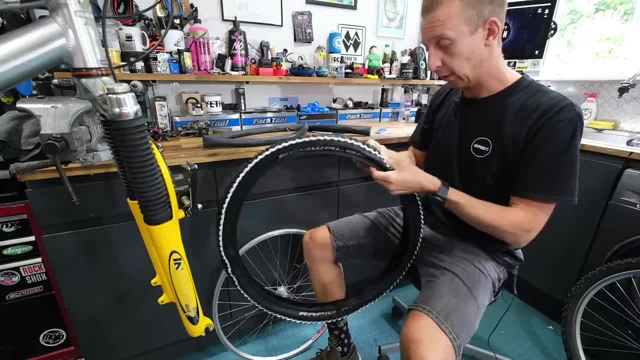 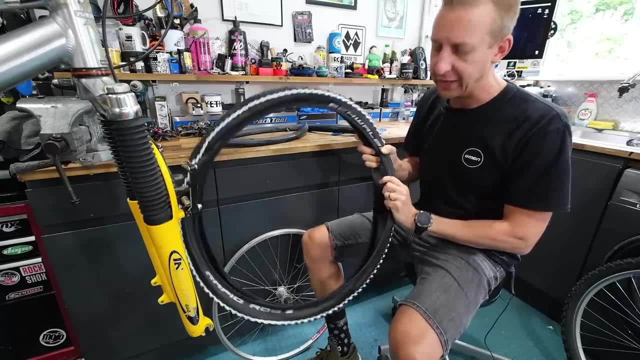 but not any longer. apparently Rapid Rob with a little white sidewall, so it looks pretty awful, to be fair. but they're cheap. Hey, I think these are about 16 quid for the pair. I got them ages ago, I think, off Wiggle or something like that. 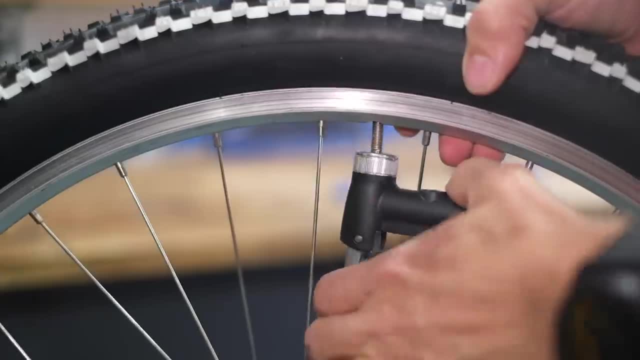 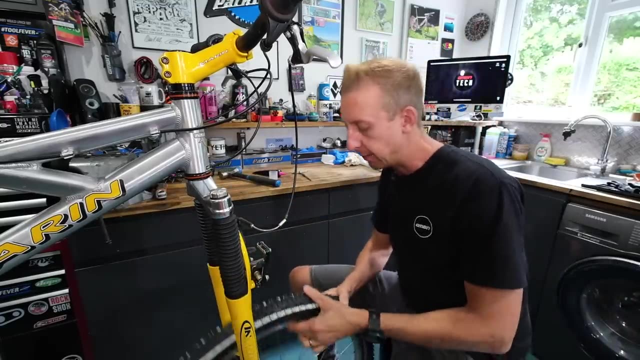 But yeah, right, so these will do to get this functioning. Let's get them on. Okay, so the fork is back in the bike. I've changed the tire on at least the front wheel for now. Time to put the front wheel back in. 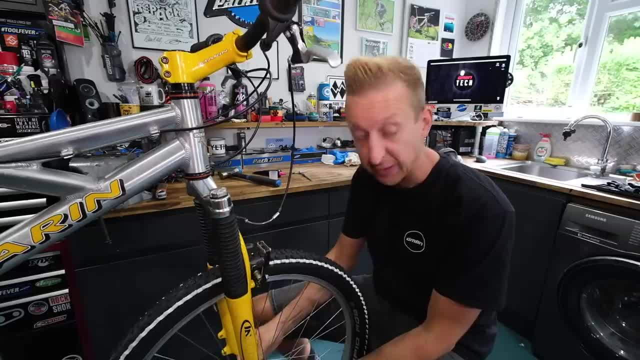 Now, before we set the brakes up, we just want to have a look at the front wheel. In fact, I should have done this just now. Just have a feel of the axle, See how it feels. Does it feel smooth, Does it feel rough? 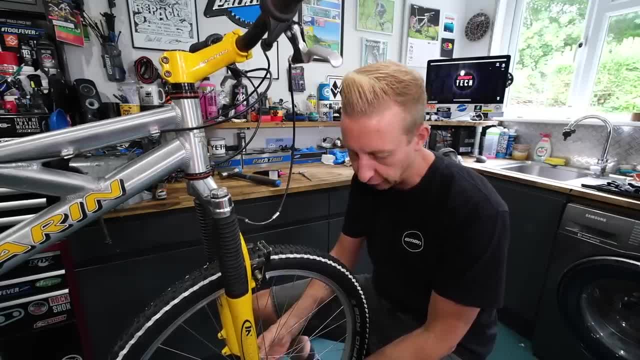 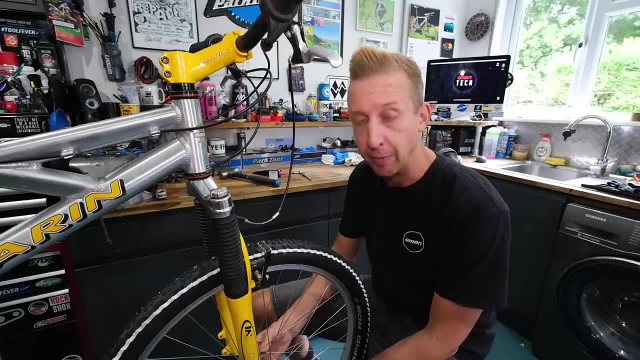 This one actually feels really smooth and it has got massive rubber seals so it looks like an old Shimano Parallax hub. It's unnamed so I don't know what it is. If it is a Parallax hub, they're pretty much fit and forget forever. 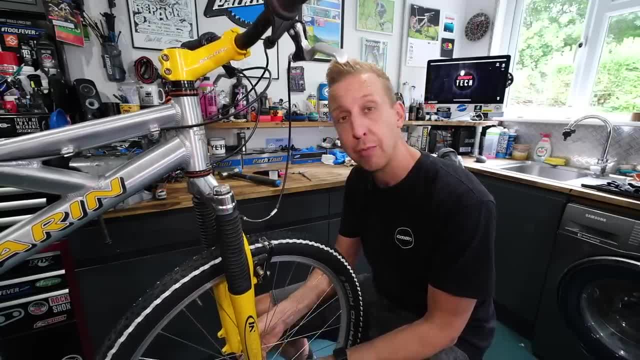 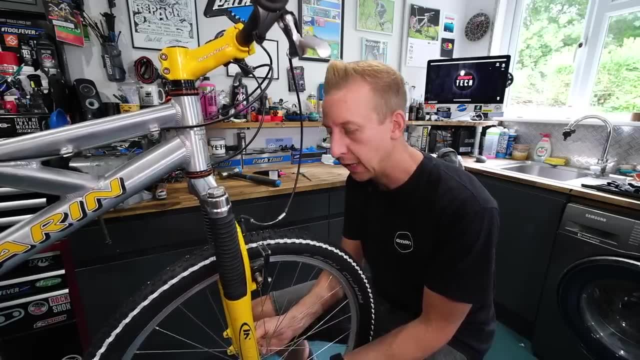 but yours might not feel like it. If that's the case, you may want to remove the axle to give it a bit of TLC. but this one is fine. I'm not going to interrupt it, Let's just get the wheel back in. 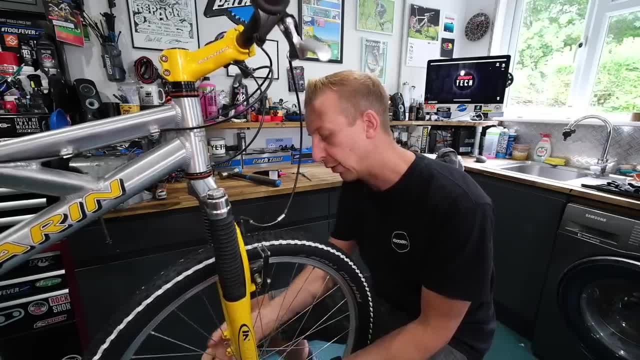 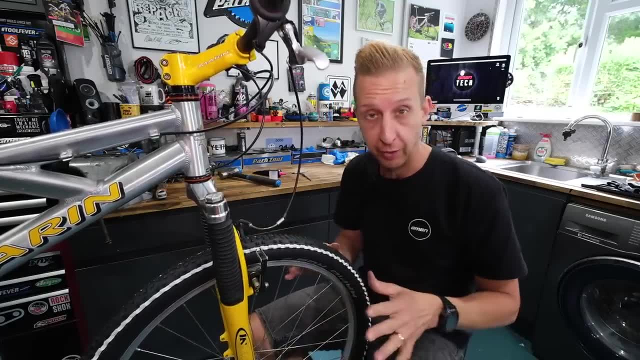 I want to make sure that the spokes are in good condition and then we can have a little safety check on the rim. Now, bearing in mind, this bike doesn't have disc brakes on it, so a lot of older bikes will not have disc brakes on it. 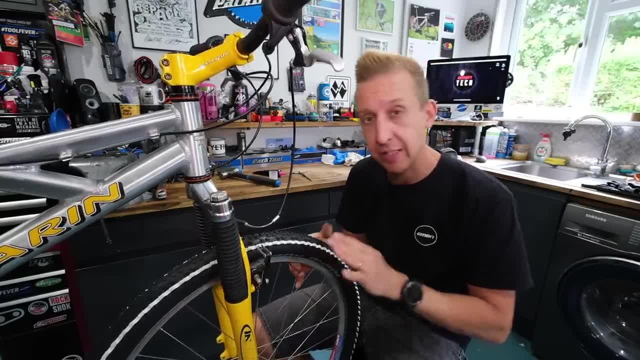 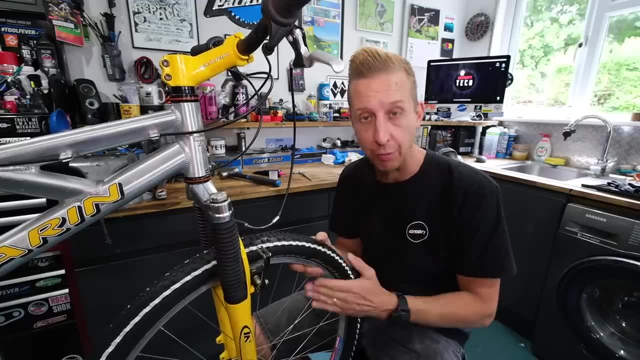 and you're using the rim basically as your braking surface. Now, this is something really important. so, bearing in mind that this is a structural part of the bike, this is a part of the wheel. you're also wearing it out by braking on it. 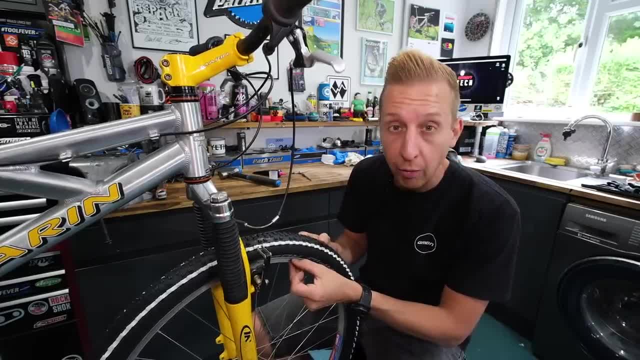 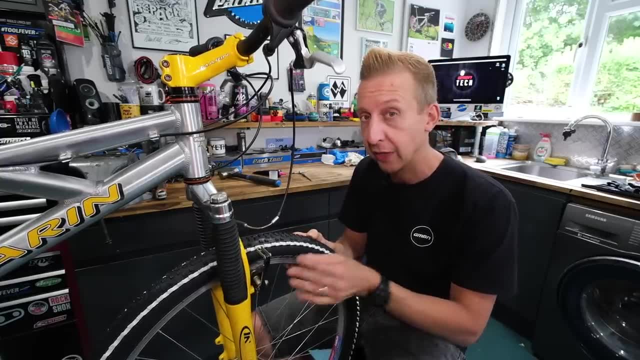 So if the bike is extremely old, if you run your thumbnail, you will actually be able to feel if the rim is pitted. If it's heavily pitted, then you might want to consider if you want to continue using that wheel. This one's just got some minor scoring on it. 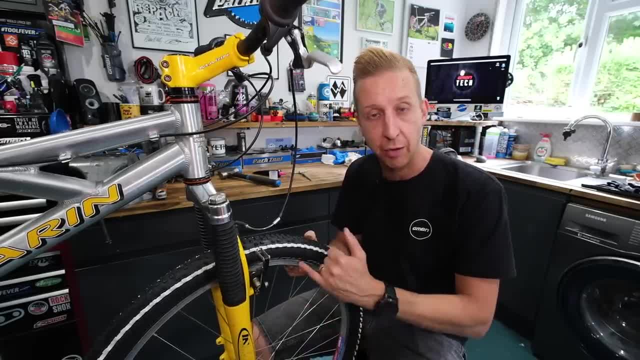 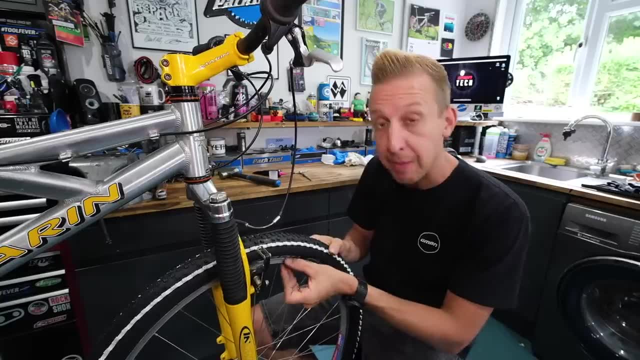 I think it's absolutely fine. but in extreme cases it's known that the sidewalls of the rims actually can break. They can actually break as well as when you're braking on them, because they're so old and perished. so just be mindful of the condition of the sidewalls. 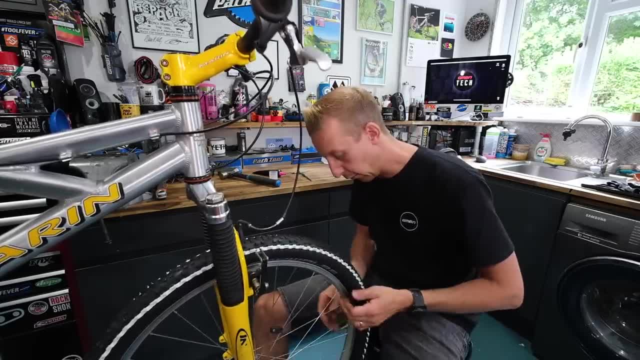 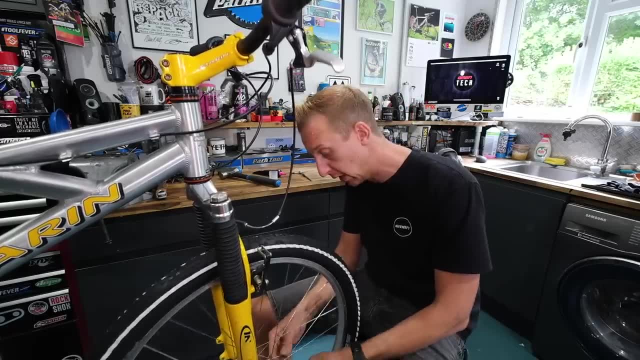 Okay. so I'm just going to run find the valve which is here and I'm just going to give it a little bit of a spoke check. I'm just looking for anything extremely or extraordinarily loose or tight. So far not too bad. 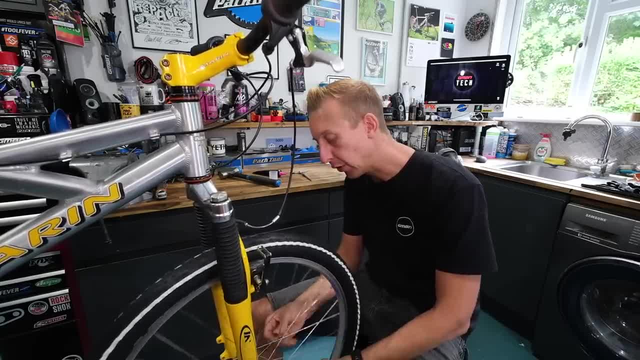 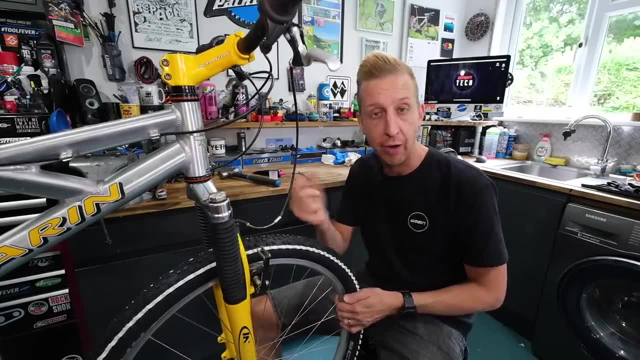 Now, if there's anything that is literally hanging apart loose and you're not someone that knows about truing wheels, you can still nip that up, but don't go too tight. Nip it up tight and then maybe another half a turn and then hopefully that won't affect things. 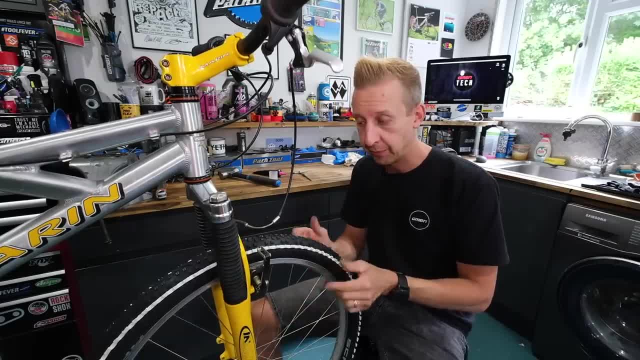 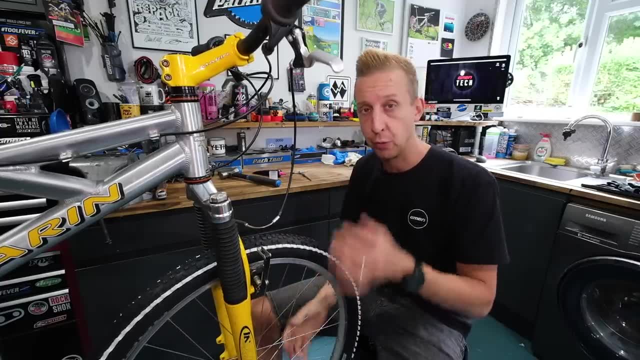 The secret with truing wheels is to do little, not to do too much, because as well as being able to pull the rim over to each side using tightness on them, you'll actually pull the rim up and down as well. So it's important if you've got a spoke. 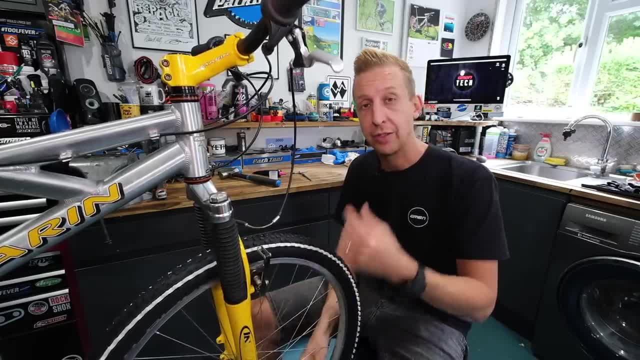 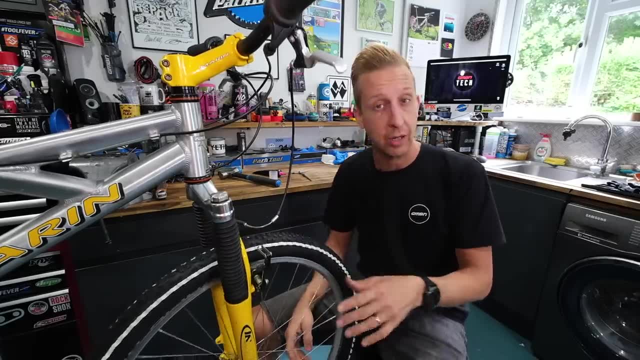 that's particularly tight, but you need the rim to move that way. you need to consider tightening on the other side and loosening that one to counter that. So there's a bit of back and forth with doing that. but if that's something you're not comfortable with, 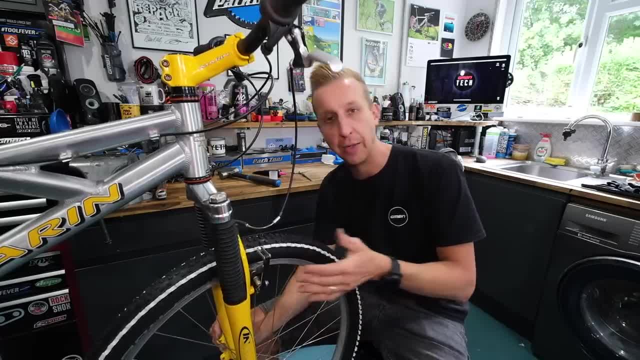 don't worry about it. As long as your wheels are loosely round, you're fine. The whole point of this is to get the bike rideable, not to make sure it's perfect. So I'm happy with those and I'm going to reconnect. 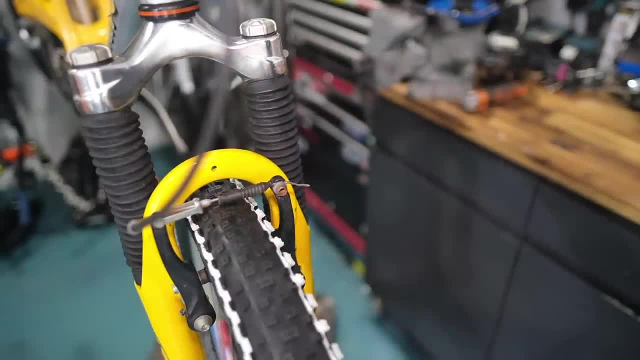 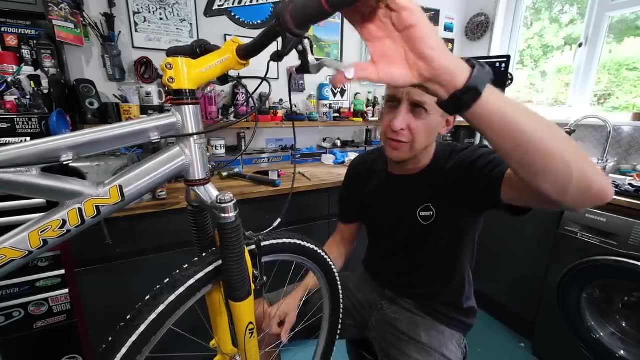 that front brake and then we're going to do a bit of work on the rear brake Right, so the brake's pulling quite far to the bars. So, and actually it felt a bit stiffer, it didn't feel too bad now. 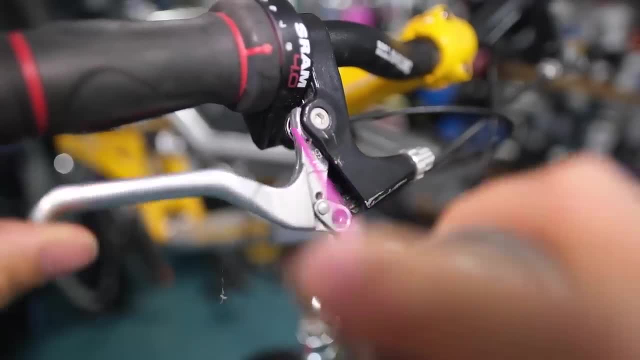 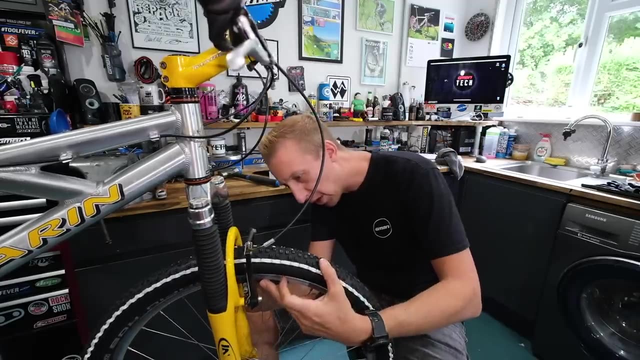 I might put a bit of lube through the brake lever there just to make sure it runs a bit smoother. And then I'm going to be looking at these brake pads Now, the front ones, I noticed they're not in the worst condition, they're okay. 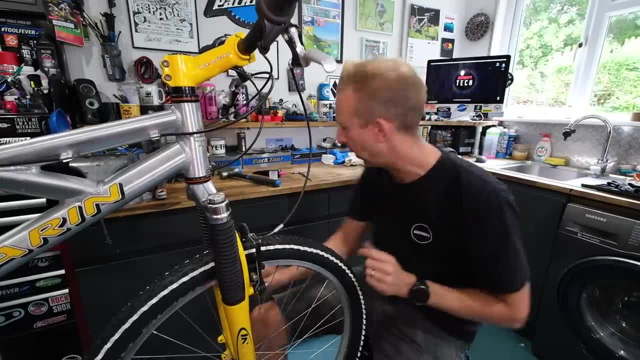 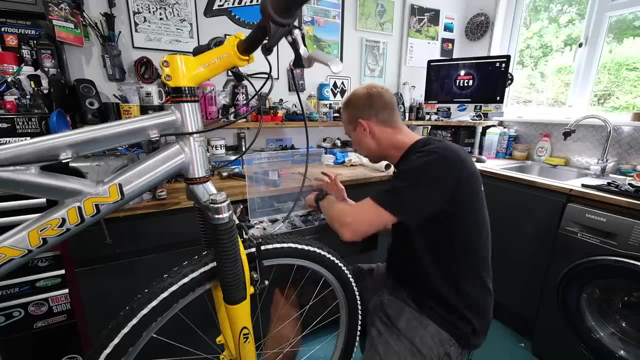 but the rear ones are caught a glimpse in the motor. they look horrendous. So we're going to change those rear brake pads. I have somewhere in one of these some old, quite the same. yeah, here we go. They're a bit smaller. so if you look at them side by side, 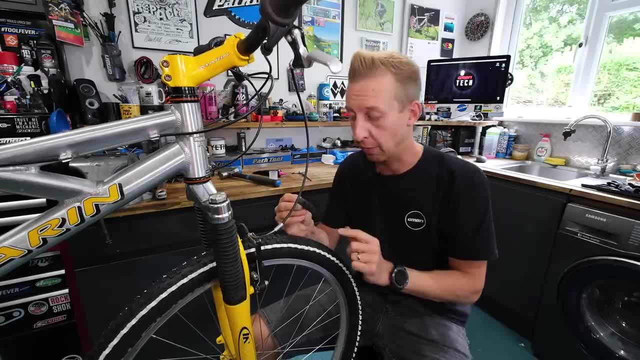 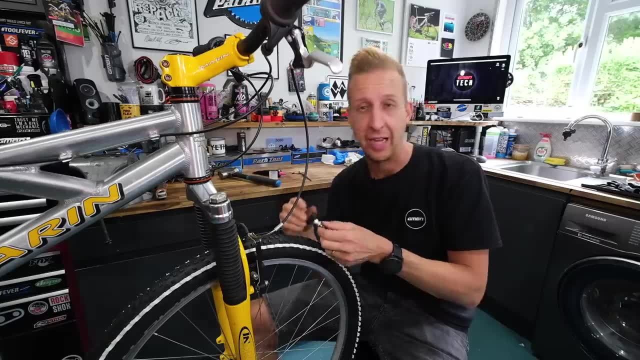 they're a little bit smaller but they've got the same fitting so we can make these work. that's no problem at all. They're just cheap old brake pads. If you do need to buy brake pads for brakes like this, for a complete set you'd be looking under 10 quid. 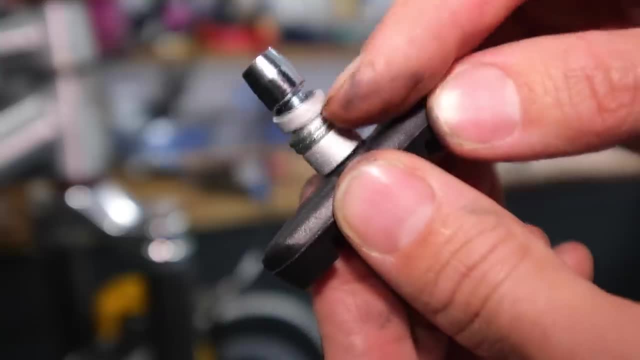 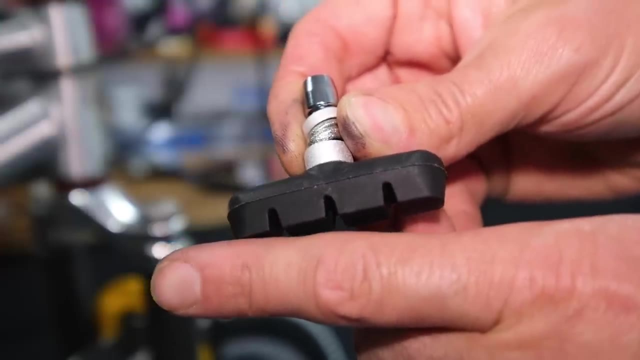 Probably five quid. if you look around Now you'll see they've got conical washers on the pads. That is so you can actually manipulate the pad back and forth, up and down, and at an angle There's a thing called toe-in. toe-in is what you want to have. 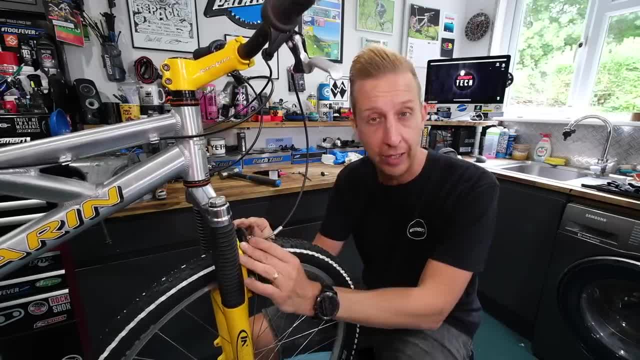 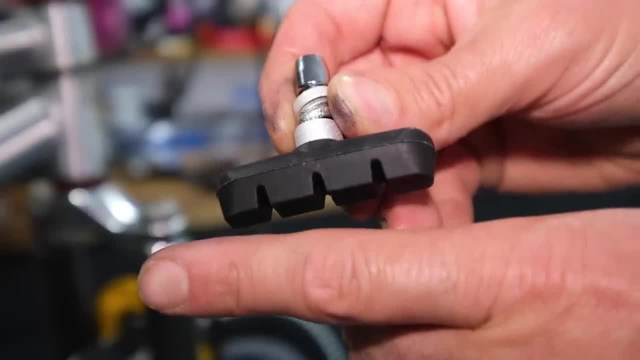 on both your front and rear brake pads. whether you have V-brakes or cantilever brakes, it's the same principle And the idea is the front of the brake pad hits the rim very fractionally before the rear does, and as the rotation of the rim goes around, 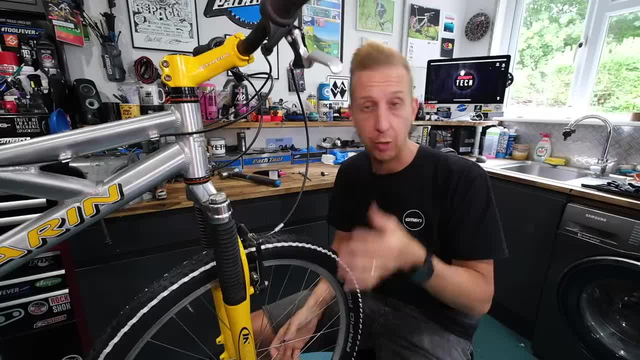 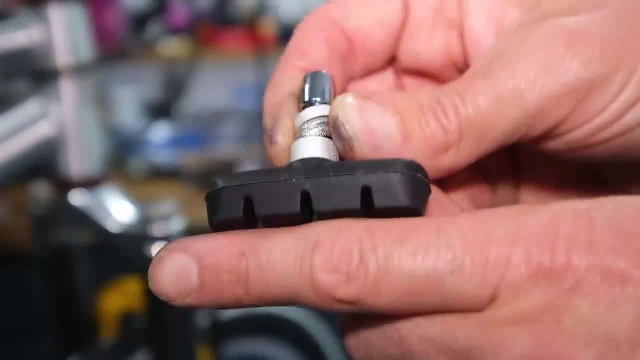 the brake is pulled onto the rim. This, in theory, helps them stop squeaking. Squeaking brakes comes from brake pads vibrating and if they hit rear first or they hit flat as they get pulled, they can go and the oscillation turns into horrendous squeaking. 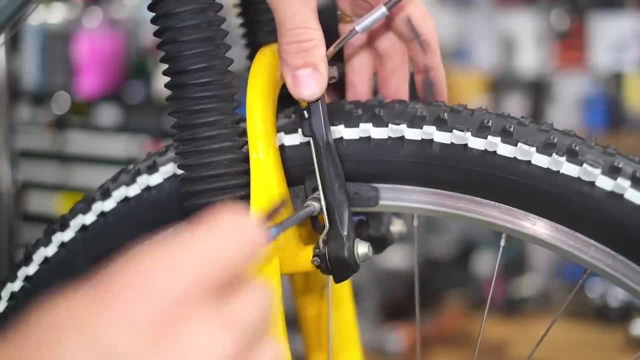 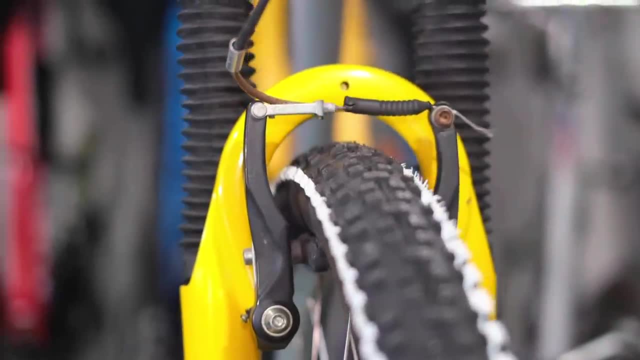 So nine times out of 10, that's what causes squeaky brakes. so get them towed in. Note that when I pull the brake lever here, once the brake pads are aligned, you can see that one of the brake arms is moving more than the other. 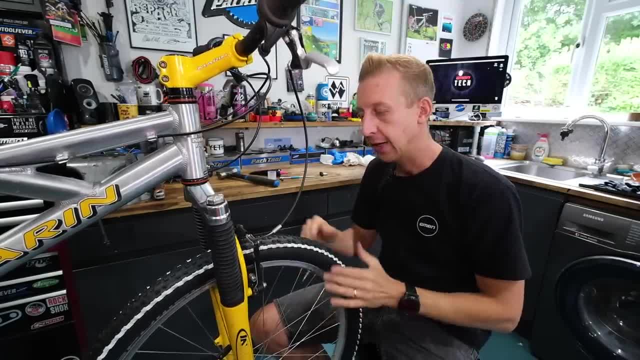 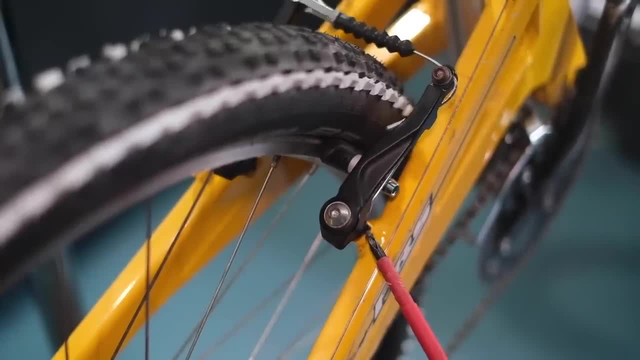 and the wheel is central in the fork, so there's no problem with that. Now they both have independent springs and, as you can see, they've got little adjuster screws here. Now these are different on all V-brakes, but essentially they work exactly the same. 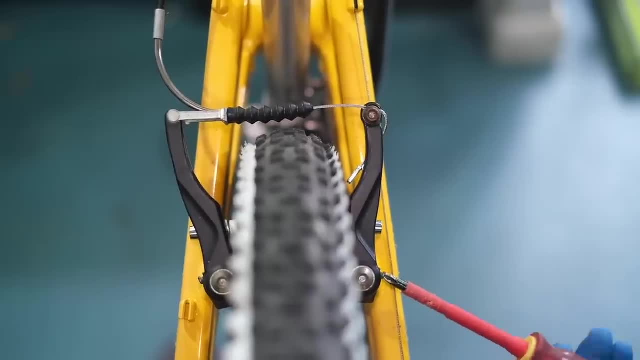 On the posh ones, you might have Allen keys. these ones are just screw heads. they're quite crude but they do the job absolutely fine. Now, just like adjusting spokes, don't think that you've just constantly got to tighten one up. 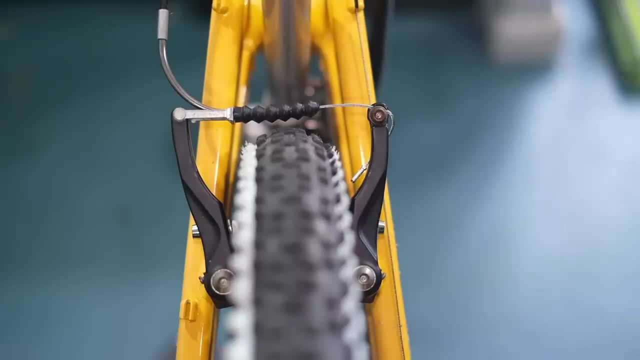 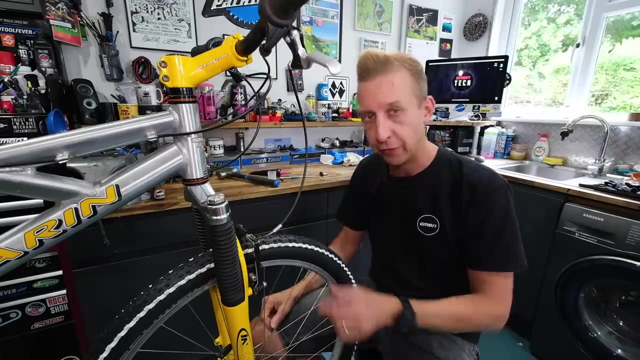 to have an effect. Sometimes it's better to loosen the opposite one than it is to tighten the one that's the culprit. Just sit back and think about it first. If it's already extremely tight, then there's a problem. You might want to back it off. 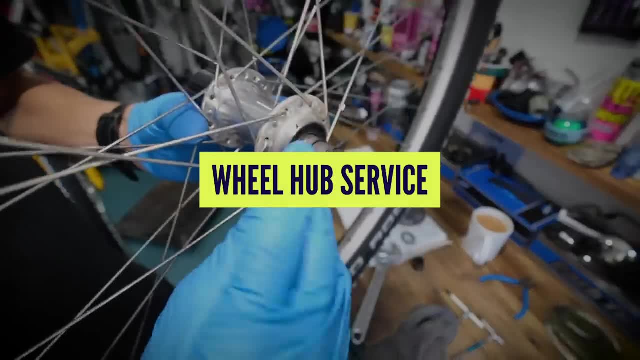 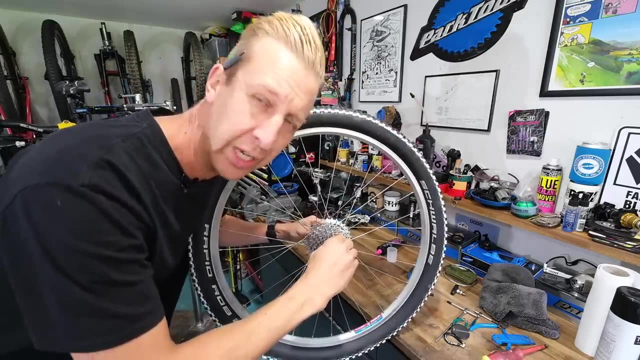 and then adjust the other one. Okay, just a quick sidetrack here. I've put the tire on the back wheel. it's all clean, ready to go. I've just noticed that the hub is a little bit grungy. 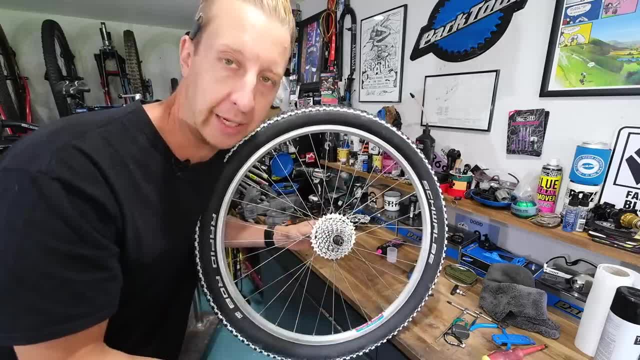 Now this isn't something that you absolutely have to do. the idea is we're getting the bike out of the shed, fixing it up. good to ride. This is fine to ride. there's no play. it does move, but I'm a sucker for detail. 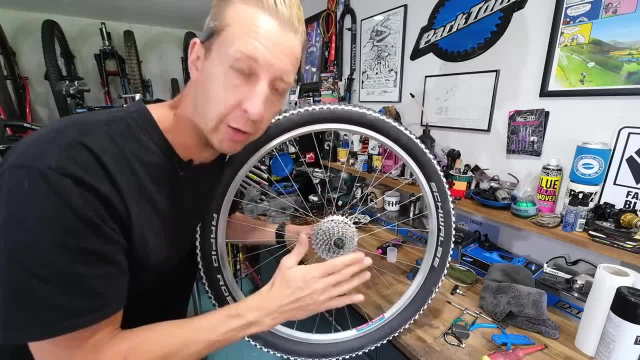 so I'm actually going to whip this out, put a bit of fresh grease in here, just so. I know that whatever we do with this bike, it's good to go Now. if you want to do that at home, you might need a few specialist tools. 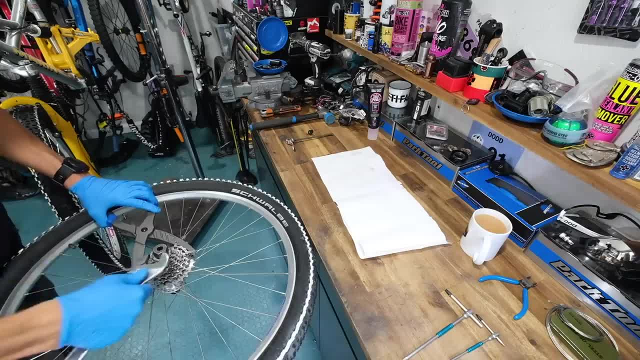 so this could slow you down a bit. You'll need to remove the cassette in order to do that, so you'll need a chain whip and a cassette tool. If you haven't got one, you can't really get the cassette off. Also, you might need some cone spanners. 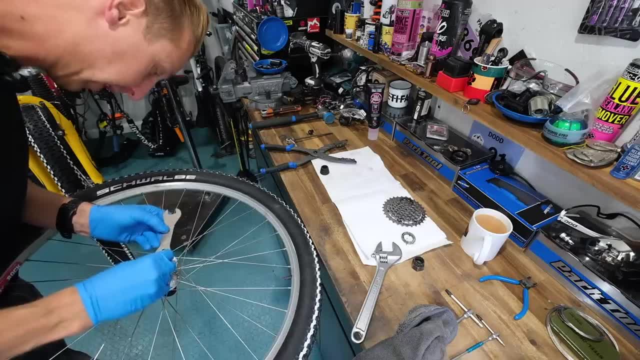 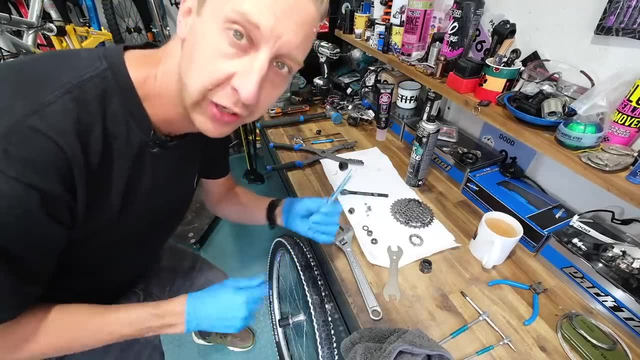 They're essentially like normal spanners. they're just extremely thin because you have a lock nut against the nut. that basically adjusts that bearing. So little tip for you as well. I've got some of these Park Tool picks. You get the heavily magnetic on the end. 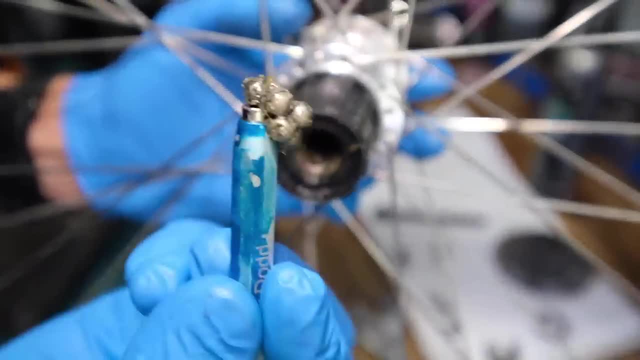 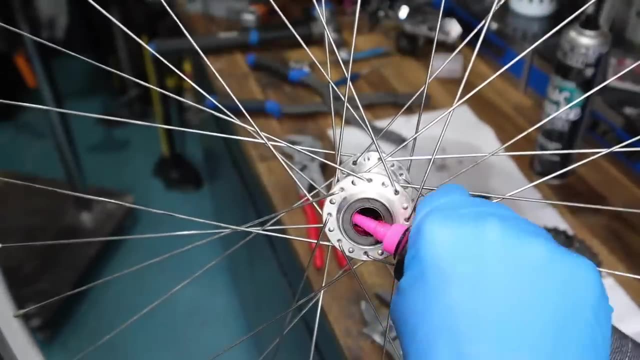 they're super good for getting out the bearings from the hub, but you can use electrical screwdrivers for that same purpose. It's got like some gunky stuff in it, so I'm just going to replace that with some fresh, nicely squeezed grease. 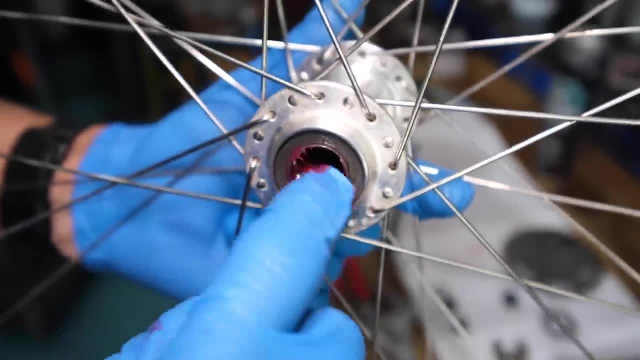 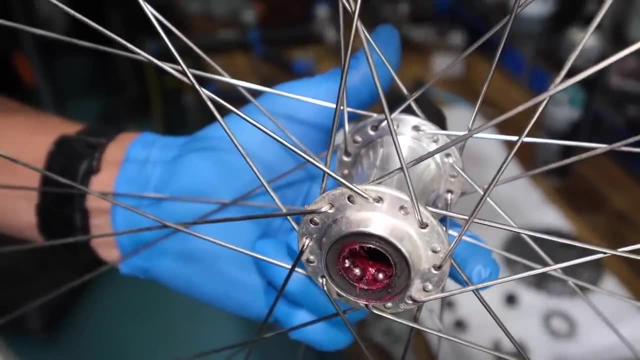 And there we go: look Nice and smooth and some nice clean grease in there. They're going to purge a bit more through, because when you put the axle back through it purges any remaining old stuff out and even to the excess stuff. 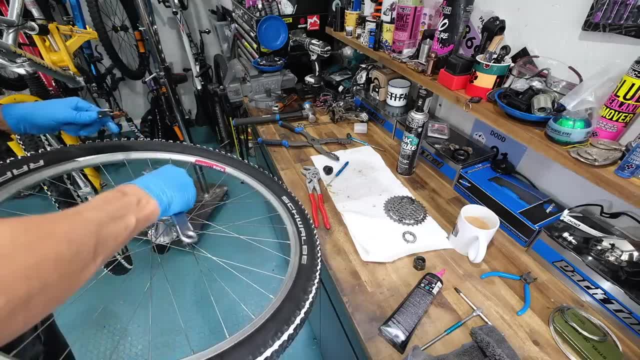 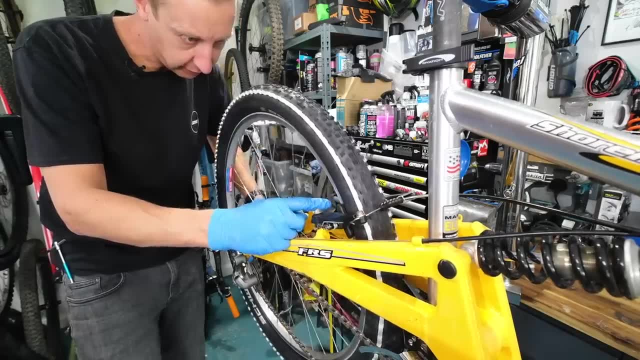 Now this hub will be good for a long time, now Sorted. I have noticed the rear rim has got a little bit of a buckle on there, so if I just feel around the spokes, you can normally feel if there's a couple that are especially tight or especially loose. 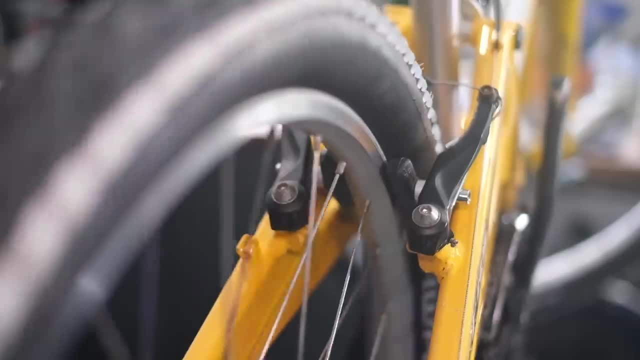 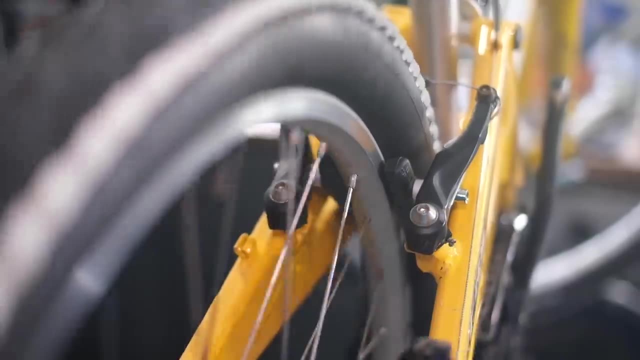 and that's normally where the culprit is. Now again, you don't need to go crazy on this, you just want to make sure it passes through smoothly enough. you don't really feel that buckle when you're braking For anything else and you're unsure about it. 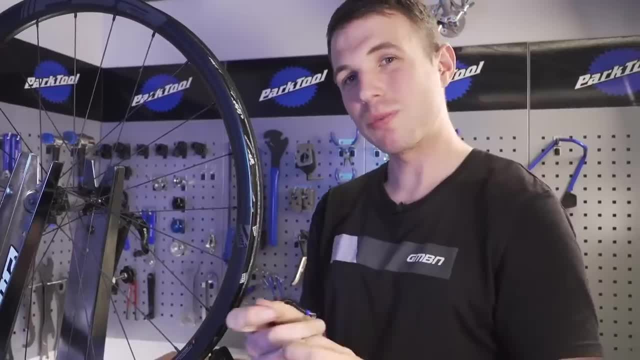 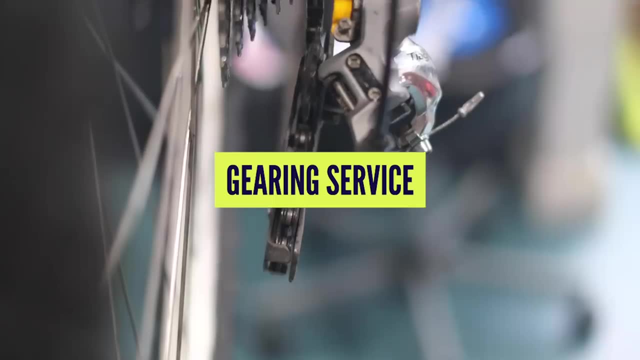 you really need to go to the bike shop to get them to true it for you. You can check our video out, but it is for slightly more competent mechanics, and that video is in the description underneath. Now let's get those gears sorted out. 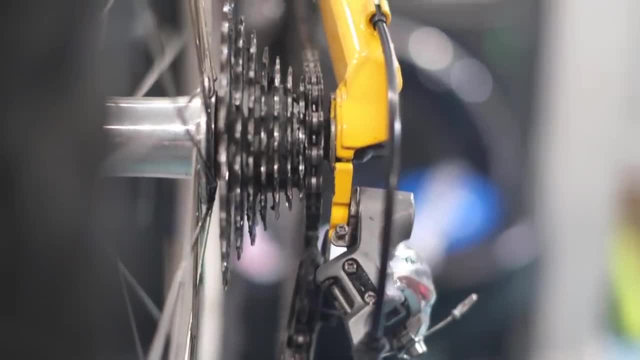 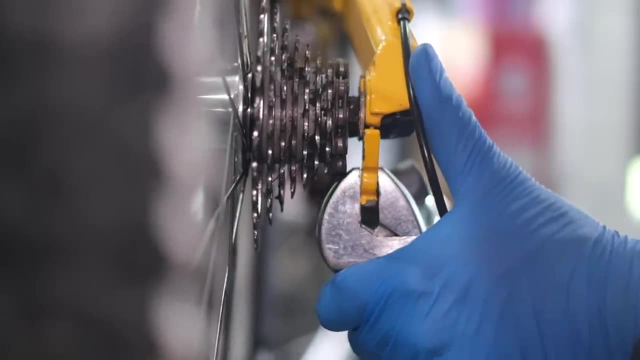 Now, as you can see, that rear mech hanger is pretty bent Right, so let's get the mech off. It's a five mil Allen key if you need to do this at home and the best thing for straightening a mech hanger. 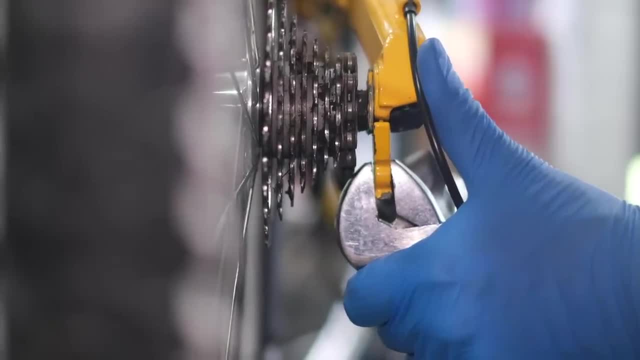 is an adjustable spanner, unless you happen to have the correct tools, but you're likely to just need an adjustable spanner here Now. be very careful with this. Some of them are part of the frame and some of them like this one. 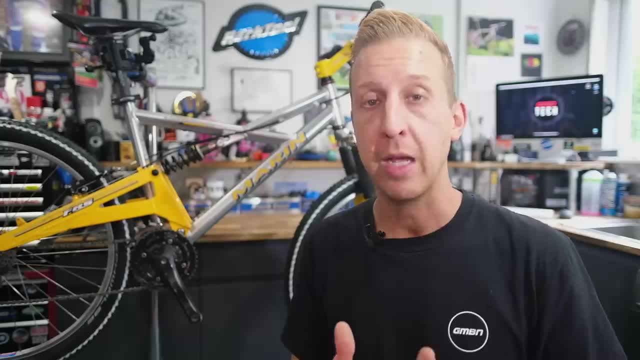 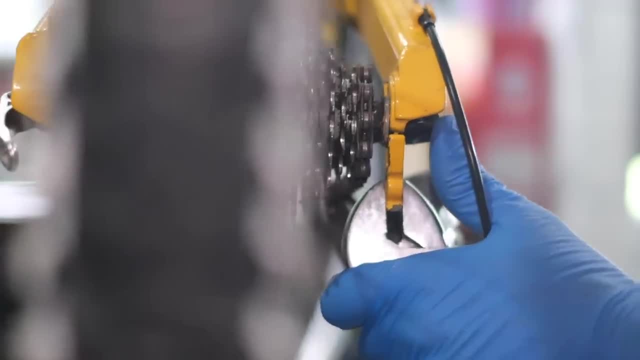 are replaceable options that bolt to the frame. Either way, they're very easy to snap and I don't want to do that. so I don't want to spend any more money on this bike than I absolutely have to. That looks okay to me. I'm happy with that. That looks near enough straight Now, thankfully, bikes with less gears- like this one it's actually- you can have a slightly more bent setup and get away with it, and you can with the more modern 10,, 11, and 12 speeds. 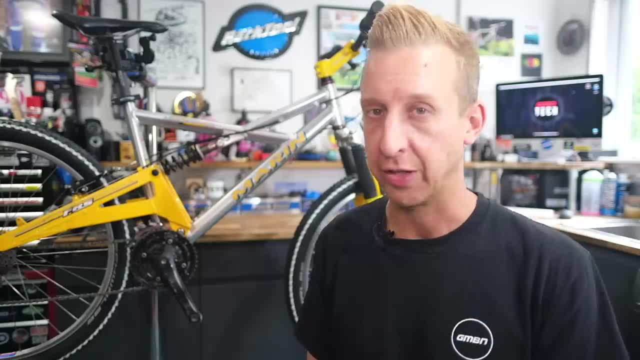 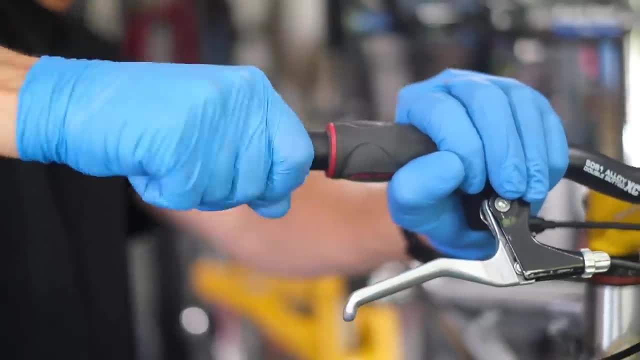 This has only got eight on the back, so this is actually quite easy to adjust. so I'm going to leave that. I'm not going to chance bending it anymore. I'm going to fit a new cable in here as well, because it's obviously had some water in the system. 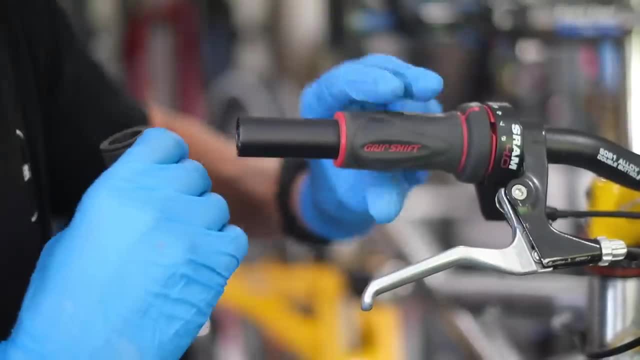 So let's get the handlebar grip off. It's only a little bit of a grip piece. We've got a grip shift. Let's take the grip shifter off. That's a little bit stiff. We'll put some suspension grease in there. 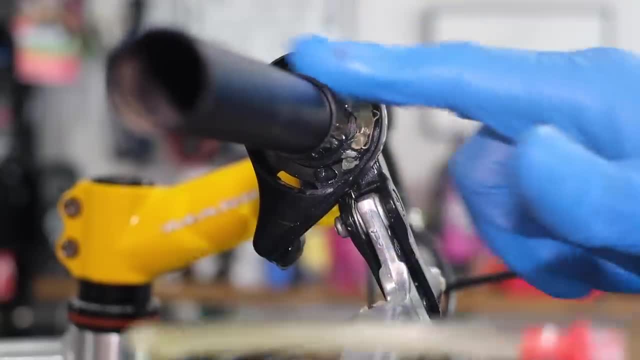 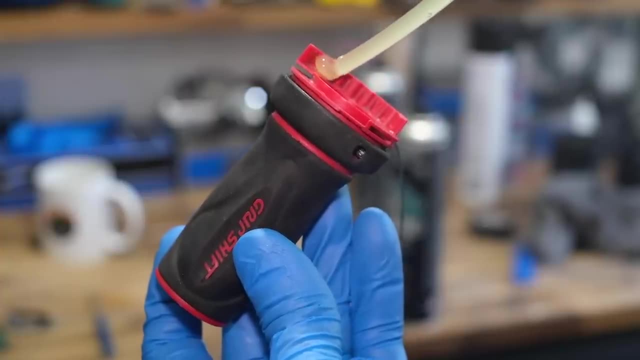 Just an important note. if you have grip shift, by the way, and you're going to put any sort of grease in them, make sure it's a grease that's friendly on plastics and rubbers. Suspension fork grease is perfect for this sort of stuff. 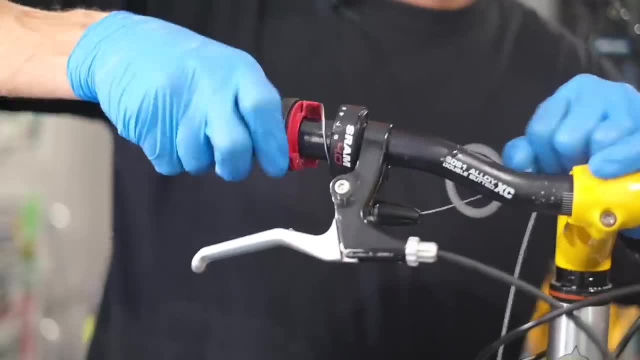 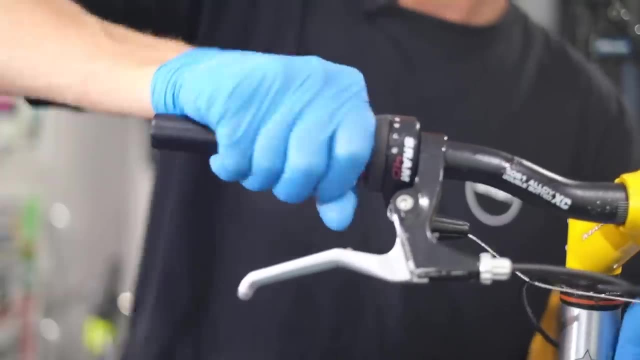 It won't deteriorate. the grip shift on the inside, New one in. Slide it back in. Just check that indexing. Yep, that feels good. Now for putting the handlebar grip back on. trust me on this one: the best thing on earth for doing that is hairspray. 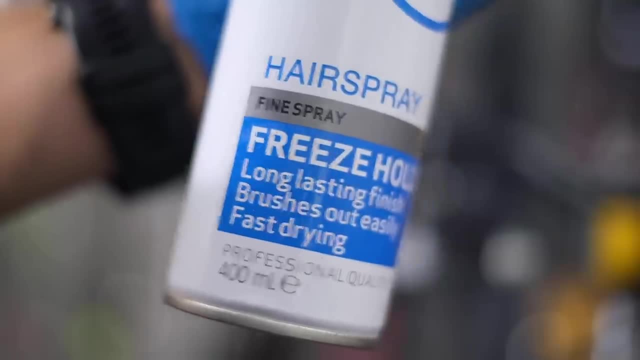 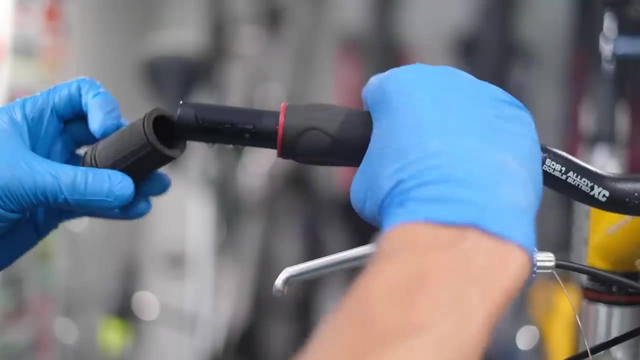 I would know about hairspray, wouldn't I? Yep, And that one is the best one- Extreme, I think it is, or something like that. It's really powerful glue. Slide the grip back on and leave it basically into its set. 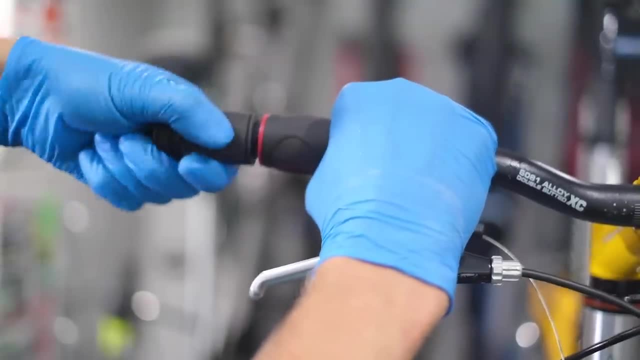 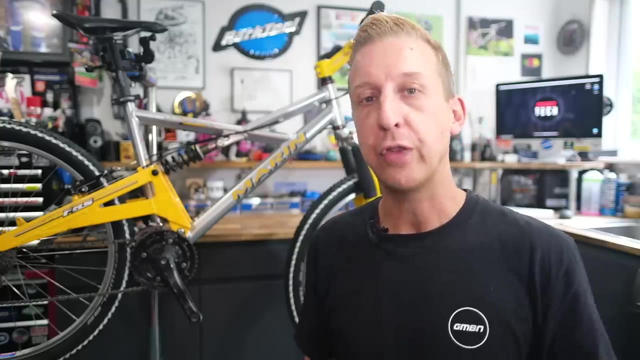 Don't be tempted to see if it's set. Just leave it As long as you can leave it, and it literally dries like glue. Brilliant stuff. Okay, so that's done. Cable back through. Nip that up Now if you do need to make any adjustments to your gears. 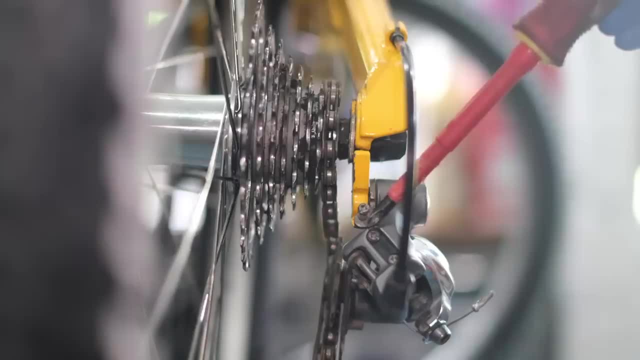 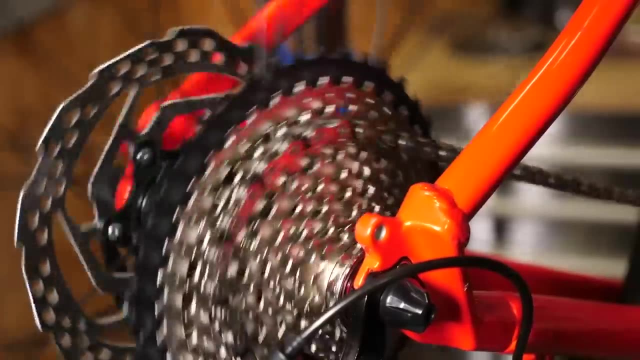 just bear in mind: there's only three real things. you need to adjust The limit. screws there they are up and down. One adjusts the inner limit, one adjusts the outer limit And then, of course, the cable tension. Now there's a video in the description underneath. 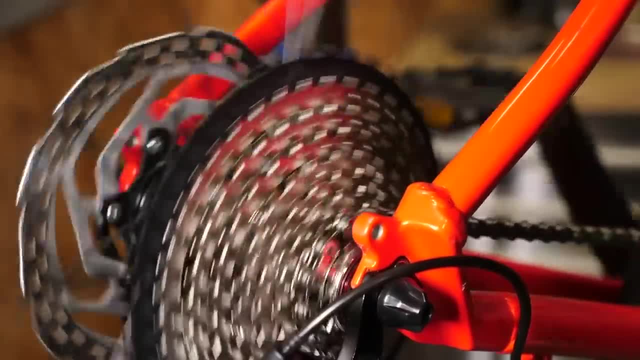 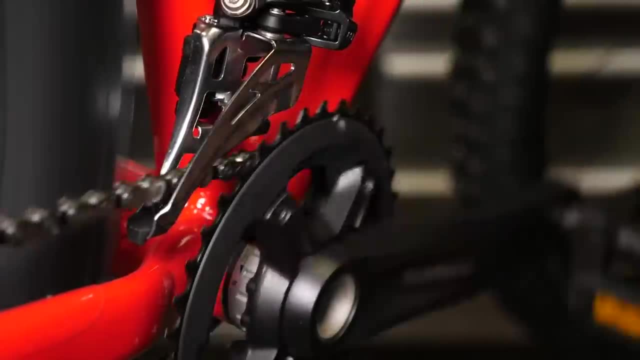 to show you all you need to know about fine tuning a rear derailleur. in the description underneath this one There's also going to be one on a front derailleur coming, so if you need to make those adjustments, there's a dedicated video for that as well. 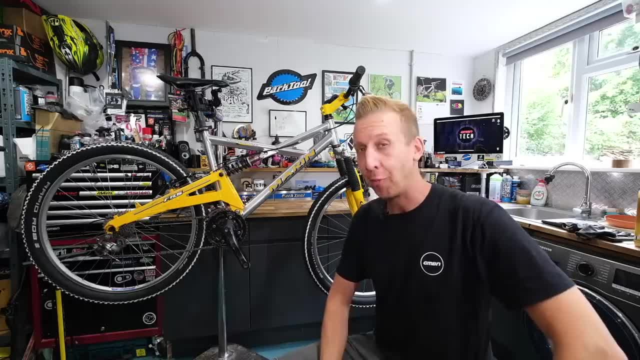 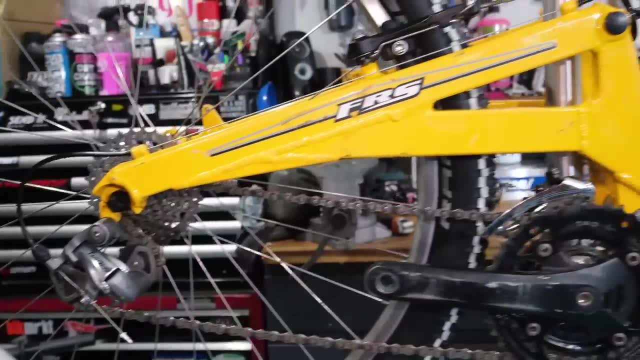 so that will help you on your way. All right, I call that a job well done. That's a old, battered up bike successfully rescued for not much money. Now the tires I did admittedly have lying around, but you could pick up dirt cheap old tires like this. 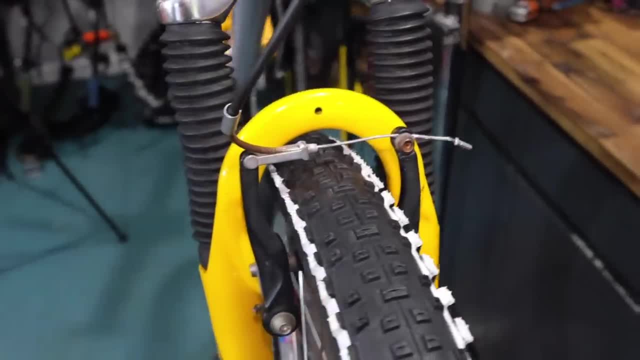 for about 10 or a piece. That's really not a lot of money and you could probably do better than these. These ones are a little bit ropey, but they will do perfectly to get the bike working. I've also put on there two inner cables. 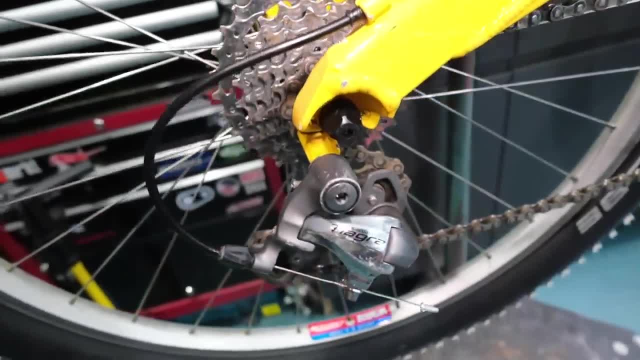 one, brake one and one gear one And again. they're dirt cheap. They're a couple of quid each. I always keep these sort of things around. Oh, I also put some brake pads on the rear. So in total, if you were to spend out on that, 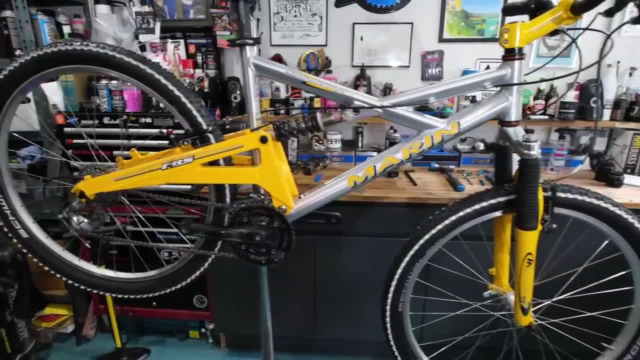 a few quid- 25 euros, something like that. that is not bad for getting a bike like this rideable again. That can make a great gift for someone. You could even sell it. make a few quid. You could definitely make a good profit on that.